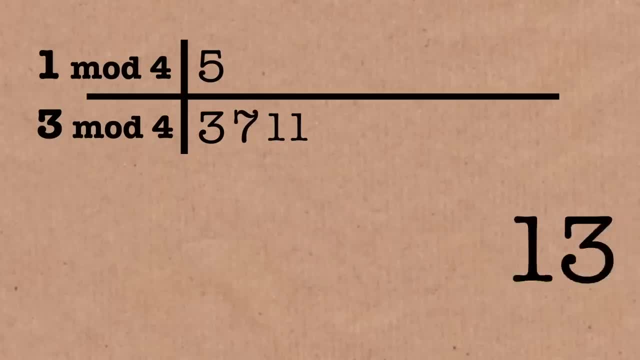 And then 11 is is also 3 above a multiple of 4.. And then the next one, 13,, is just 1 above a multiple of 4.. And then the next one 17.. So they seem pretty neck and neck, so far as we're kind of counting up. 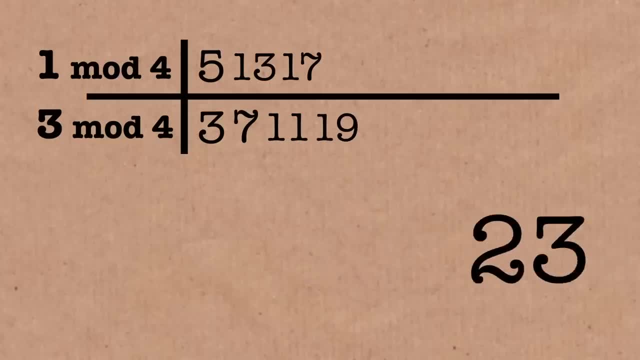 So after 17, we've got 19,, which is 3 above a multiple of 4.. And then 23,, which is 3 above a multiple of 4.. And then the next one will be 29,, and then after that we're going to have 31,, 37.. 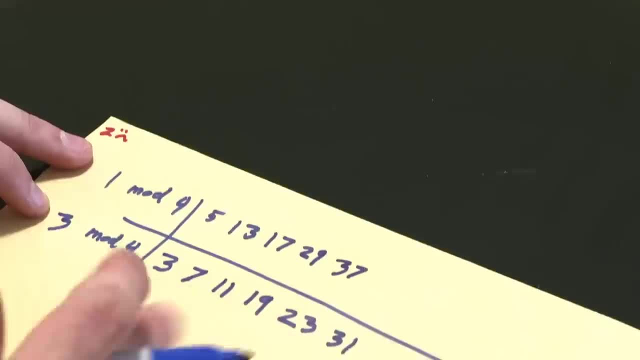 And one thing you might notice is that so far in the whole race, even though it's pretty neck and neck, Team 3 is always going to be in the lead. It's always been in the lead so far, And you might say, okay, that seems maybe just kind of at random, that that would be the case. 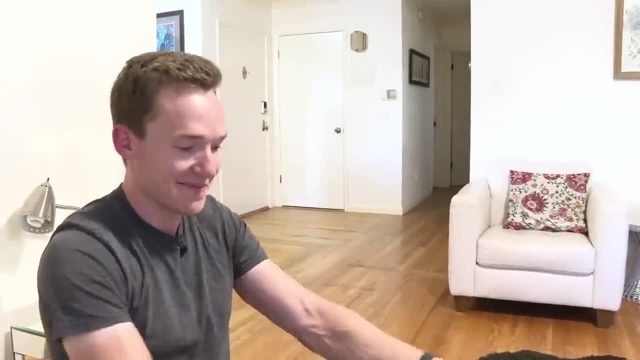 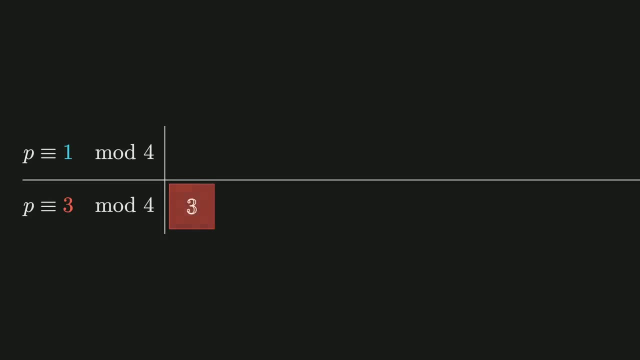 But actually, if we continue this race and if you want, I can give you some visuals that like show the race continuing on- Do you know someone who's good at making mathematical visuals? I can call a guy, But it will be. it'll always be 3 who seems to be in the lead. 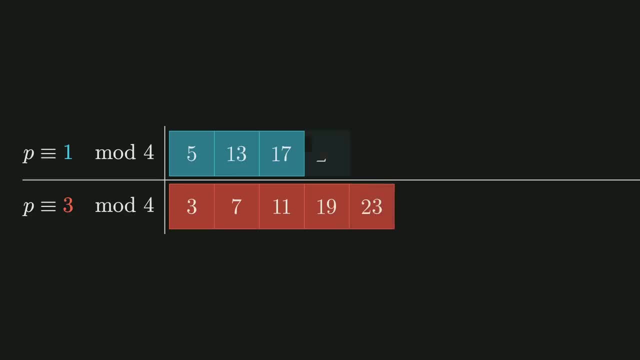 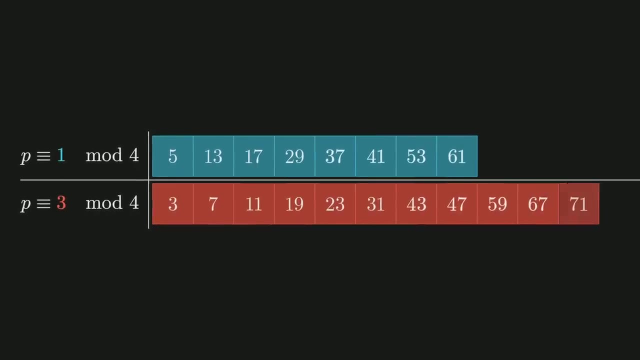 And you know they're pretty close. they're a pretty even balance, like you might expect. But if it was completely random, if it was just random, which bucket you're tossing it into? you wouldn't expect such a long streak For there to be a particular winner. 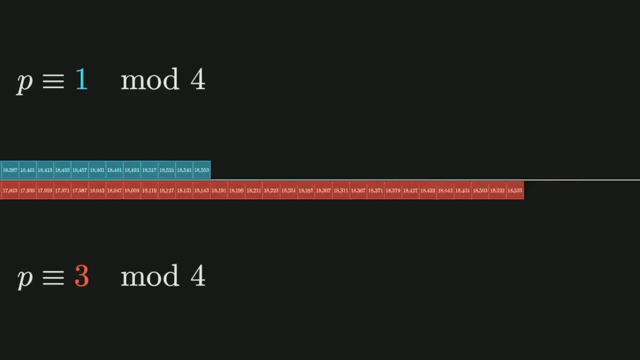 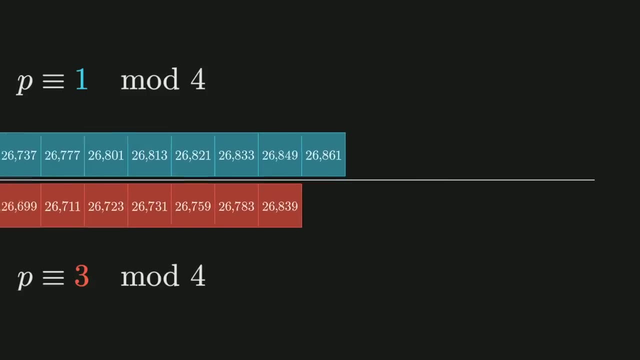 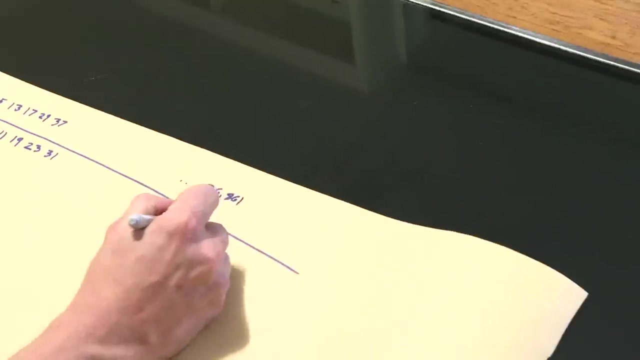 And in fact it continues going on until the first time that Team 1, Mod 4, is going to break into the lead is going to happen at the prime 26,861.. But even then, next prime after that is going to be 26,863.. 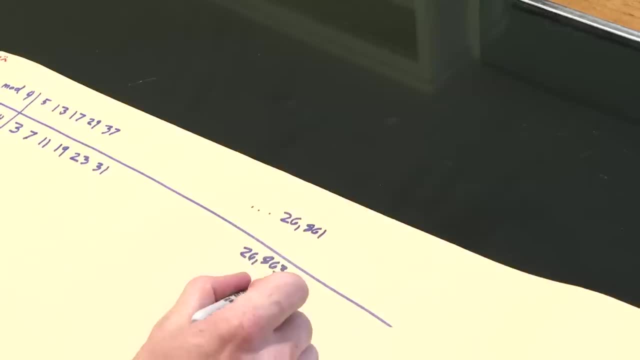 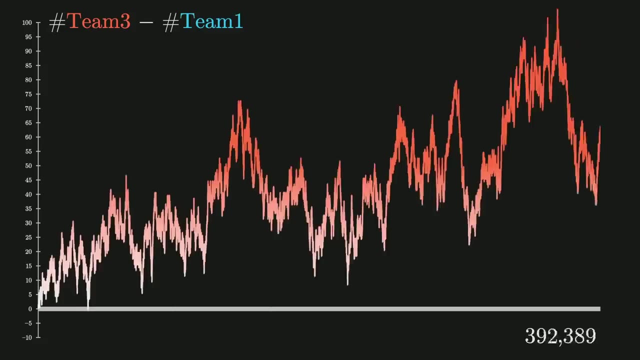 So that was just one brief moment of peeking into the lead, And then after that they do stay in the lead quite a bit longer. Team 3, Mod 4.. And then the next time the Team 1 is able to get ahead is going to happen at 616,841.. 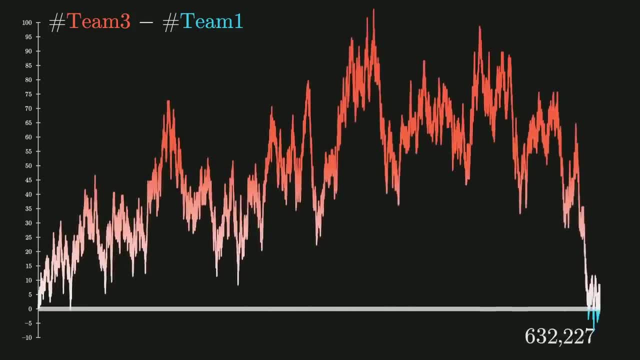 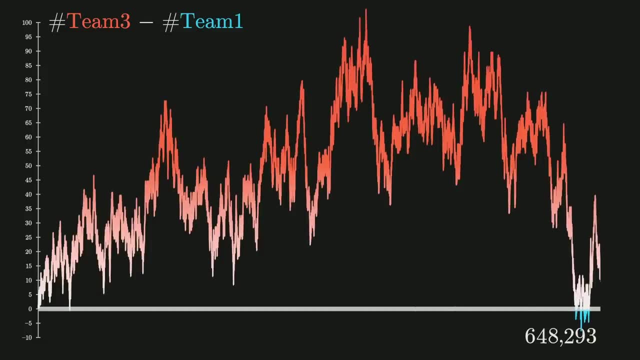 And it keeps the lead a little bit longer then. but then 3 takes over And if you're looking at most of the numbers, most of the time it seems like 99% of the time- the team that's in the lead is Team 3.. 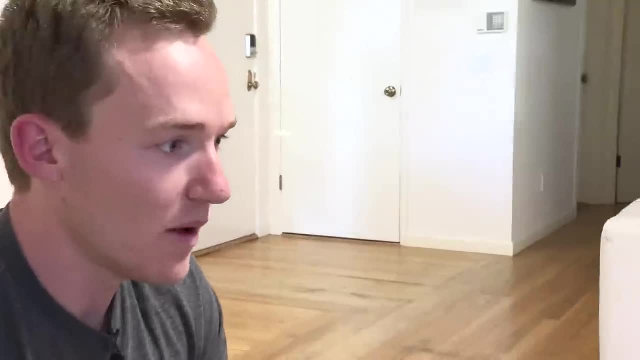 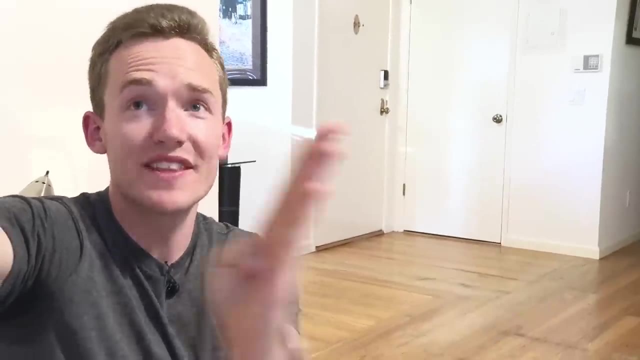 And this was actually a conjecture that someone made. that said, is it the case that, as we let n tend to infinity and we consider hey at all of the points of the race, how often was it the case that Team 3 was in the lead? 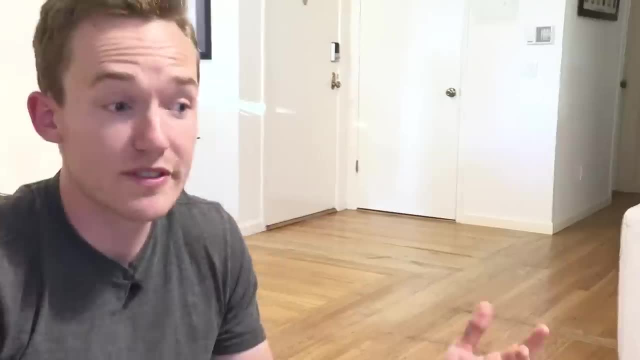 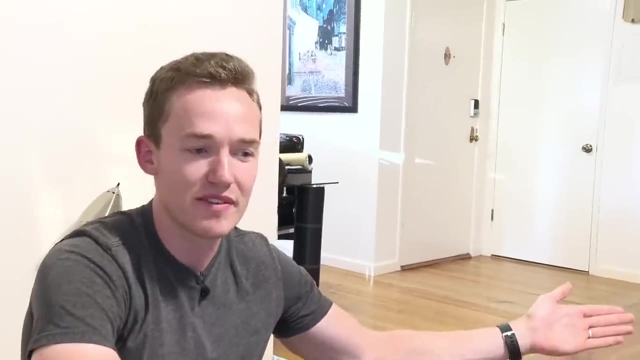 Does that percentage of the time approach 100%? Interesting question. You might expect it to be true. If there's any reason that there should be more 3s, then you might expect it to either fall- you know, completely- 50-50 or completely to 100%. 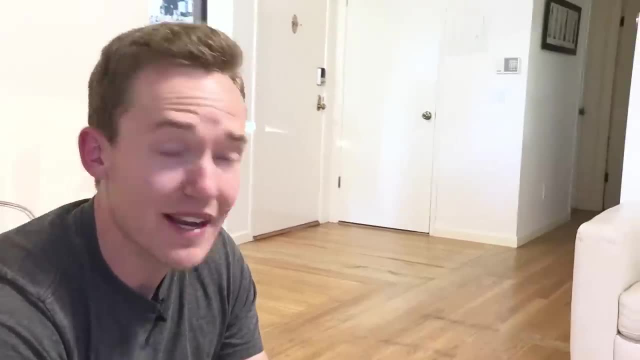 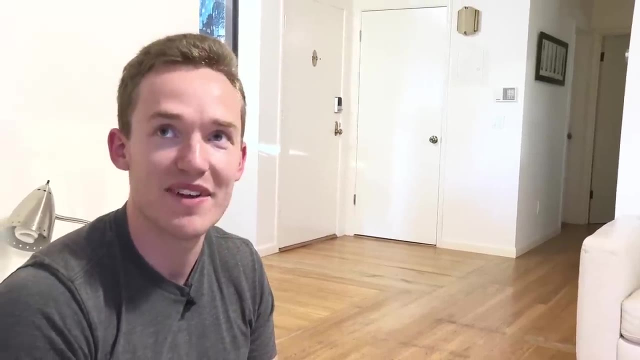 But you know, I think the question I'd like to talk about a little is: why would you expect something like this to happen? It feels like the Primes shouldn't have a bias one way or another. Why does this team get any kind of advantage? 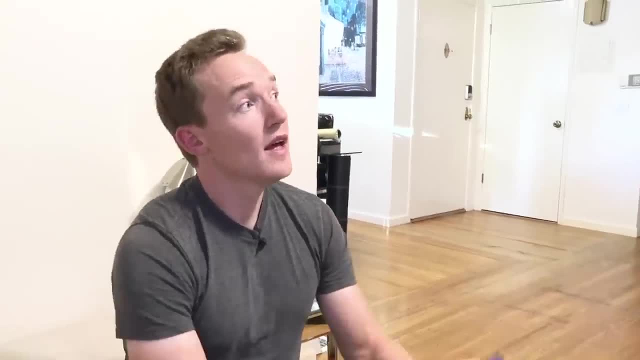 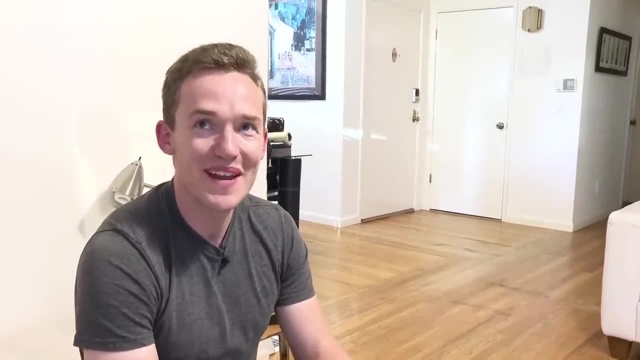 Well, Primes do have a bias. They have a bias towards odd numbers- Fair point, Okay. so there's a very strong bias towards odd numbers And maybe you're onto something there that we shouldn't treat Primes so randomly. but often you have this criteria that once you rule out the obvious things that Primes aren't 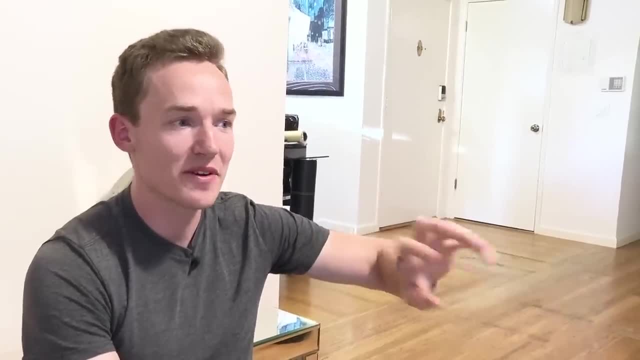 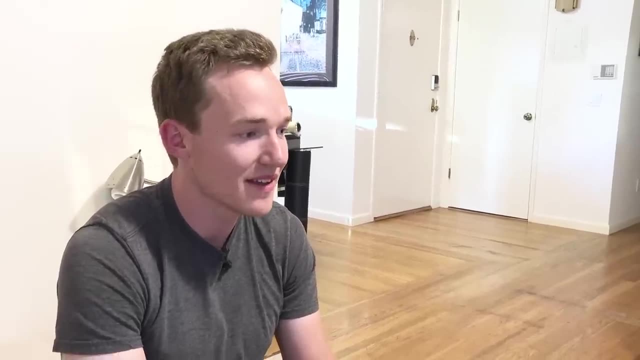 going to do the things based on divisibility constraints. their behavior feels random And this heuristic actually helps people make a lot of conjectures and a lot of it kind of susses. out turns out to be true once you delve into it. 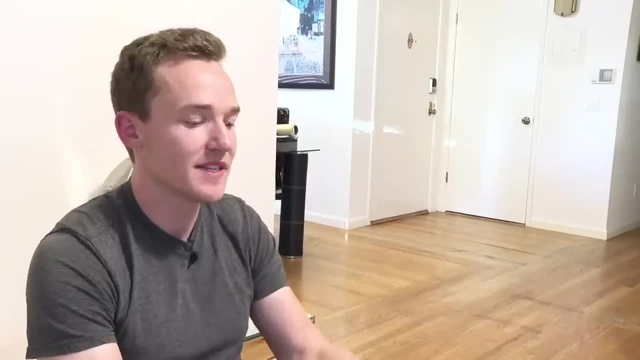 And so something like this, another one that's in the same vein. let's say, we look at the last digits of the Primes: Is it going to be a 1? Is it going to be a 3? Is it going to be a 7?? 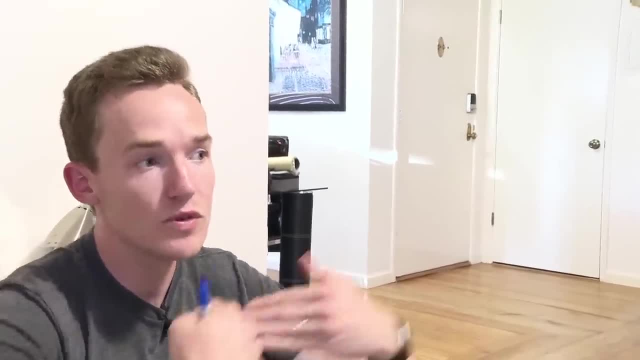 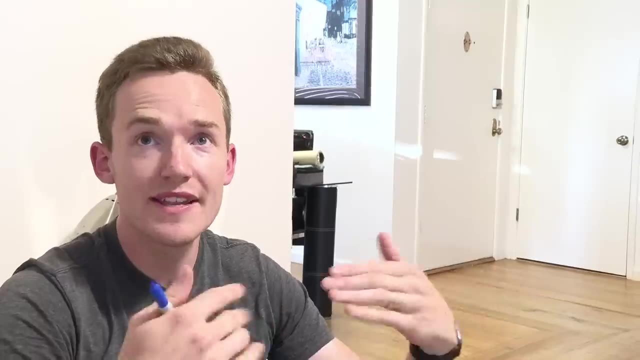 Or is it going to be a 9?? If you perform that race as you do that, longer and longer. they all tend to be about 25% of the time, but two of them are distinguished winners. They tend to be winning the race, even if it's just by a little bit. 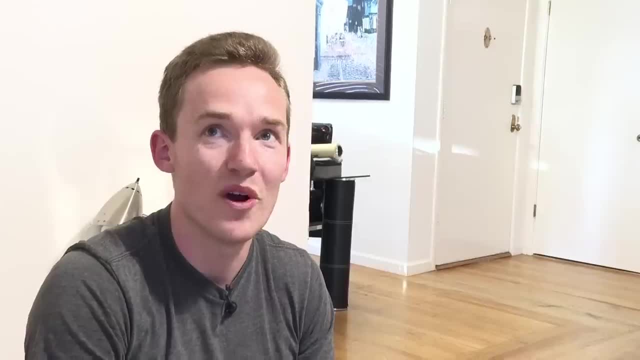 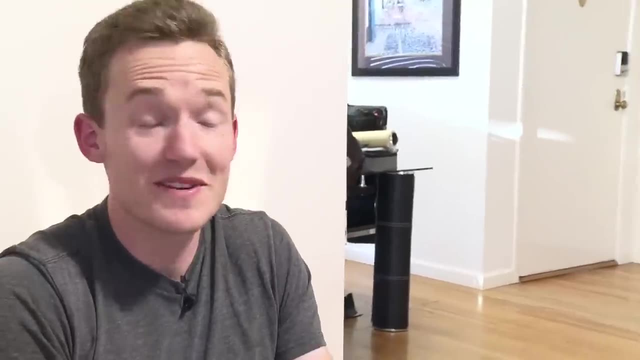 So in the long run it tends to be about 25% of the Primes end in a 1,. but there is just a gentle bias And you might ask why. Okay, you say they're biased to be odd. There's a very clear reason: they're strongly biased to be odd. 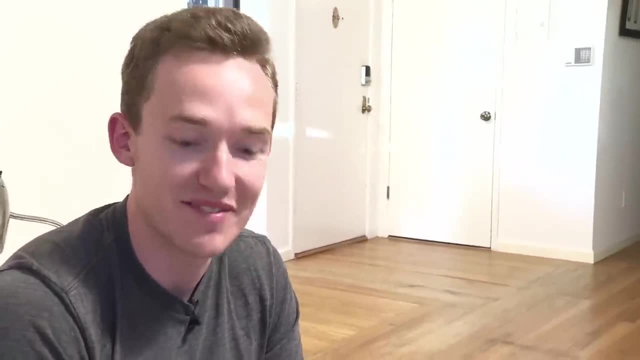 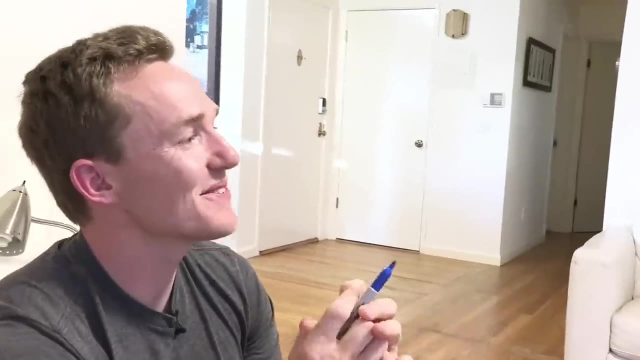 What is the reason, then, that 3 mod 4 would have this kind of advantage? So are you confirming to me that it does have an advantage? Has that conjecture been proven? That's a really interesting question which we will get to at the end of the video, actually. 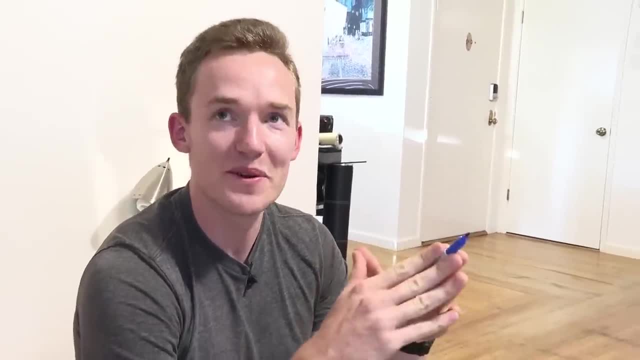 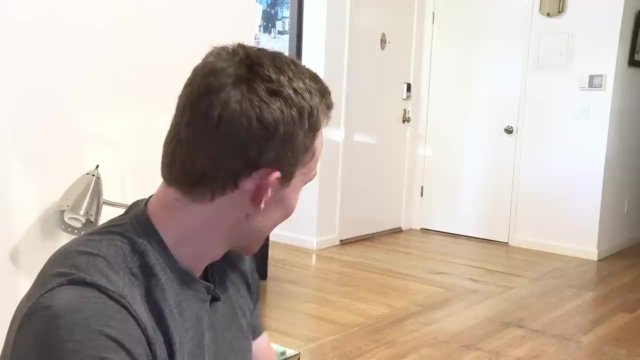 For the moment, let's just consider that conjecture, something that has strong empirical suggestiveness, but it's very tricky to prove that kind of thing, And then the answer is surprising and we will get to it. Here's a question of how much detail we want to go into. 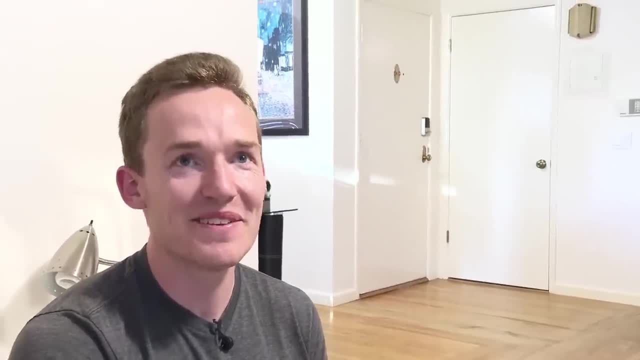 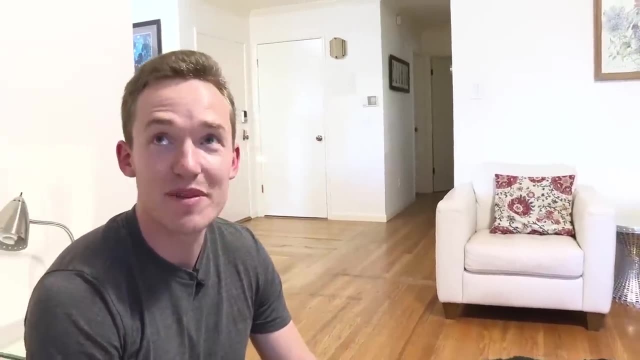 I think this is a pretty satisfying intuition if you're willing to take on faith one magical fact that I present to you. So the story is going to start outside of here, but instead with a formula a lot of people might know, for pi of all things. 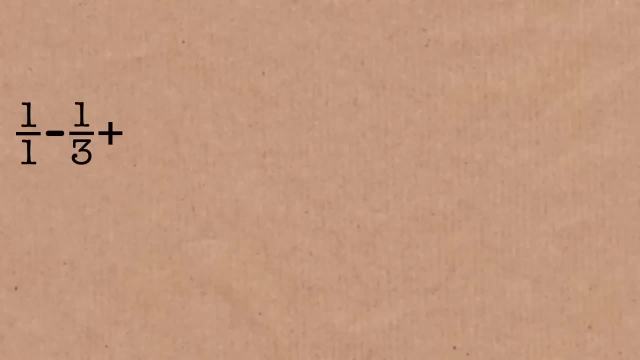 1 over 1, minus 1 over 3, plus 1 over 5 minus 1 over 7.. So I'm basically toggling whether I add or subtract and I'm going over all of the odd numbers. So this isn't primes, it's all of the odd numbers that I'm doing. 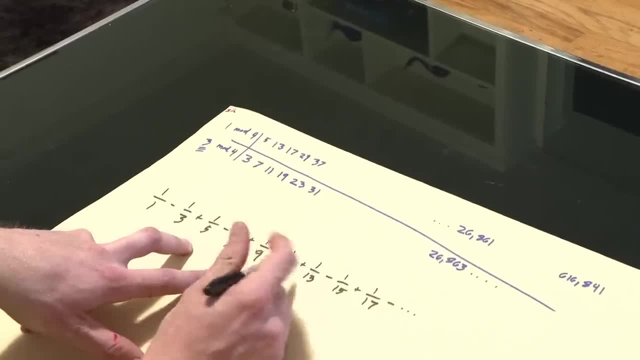 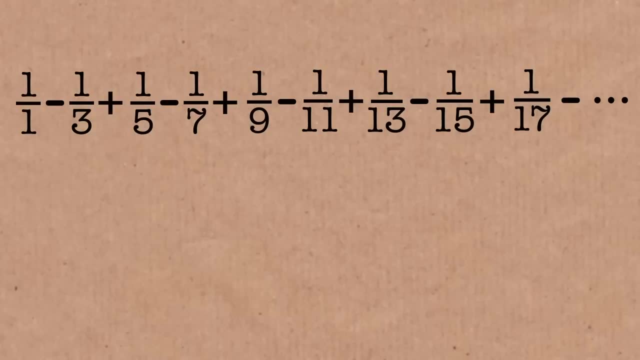 In fact I'm going to give a name, to let it be kind of clear, this plus minus pattern, where I'm going to make up a function that seems needlessly complicated right now, that I'm going to call chi of n And basically chi of n is going to be defined to be plus 1 if n is 1 mod 4.. 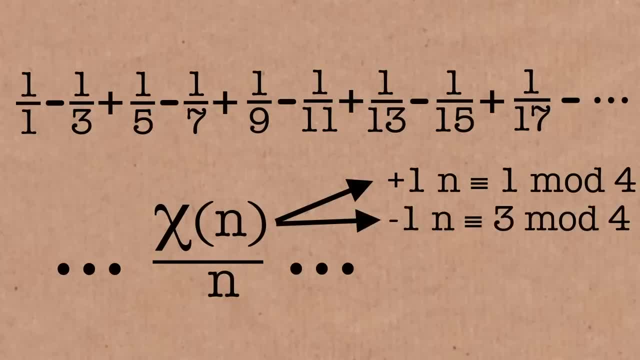 It's going to be minus 1 when n is 1.. n is 3 mod 4.. And then I could maybe say that it's 0, you know, if n is even. And so basically, what we're doing is we're adding up chi of n divided by n. 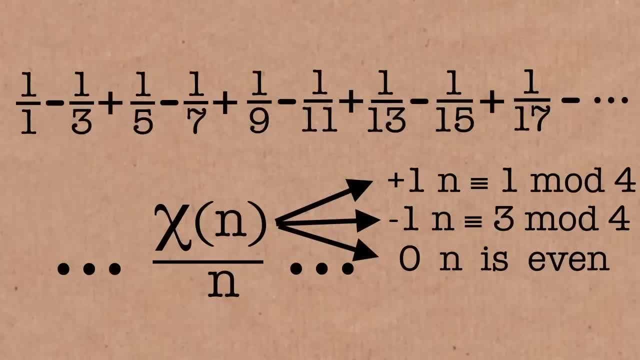 Overly fancy way of saying I'm toggling between plus and minus on the odd numbers, but it's nice to have a name for that function for what we get to in a moment. Now some people might know that this actually converges. If you look at this on the number line, you have your 1,. 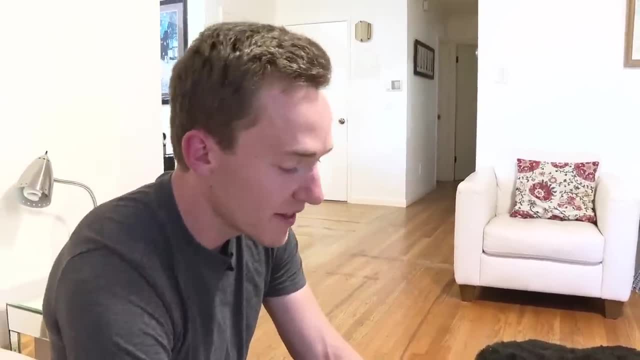 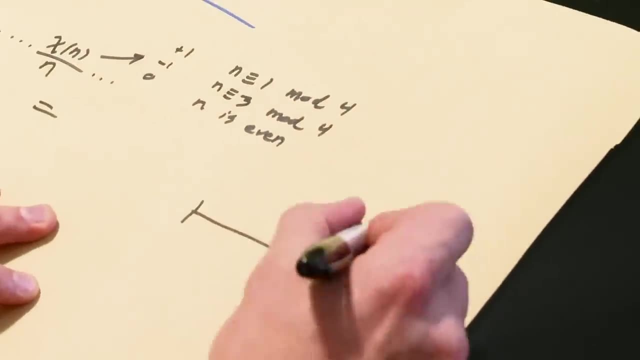 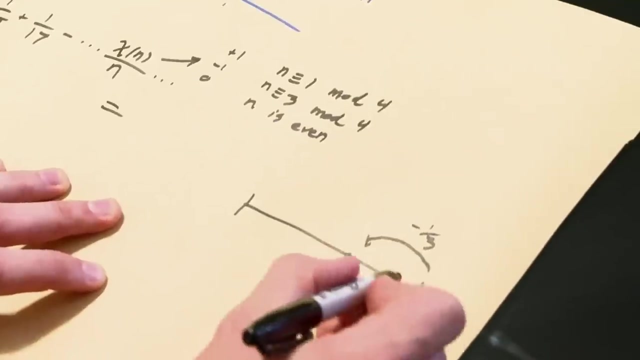 you subtract back a little bit to 1 third plus a fifth, minus a seventh, and I can even draw that out a little bit if we want, We've got 1.. If we subtract a third, you land somewhere here. If we add a fifth, you know, because that step is smaller, we don't quite get to that 1.. 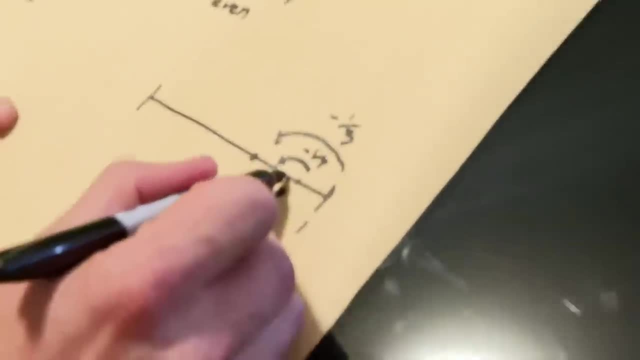 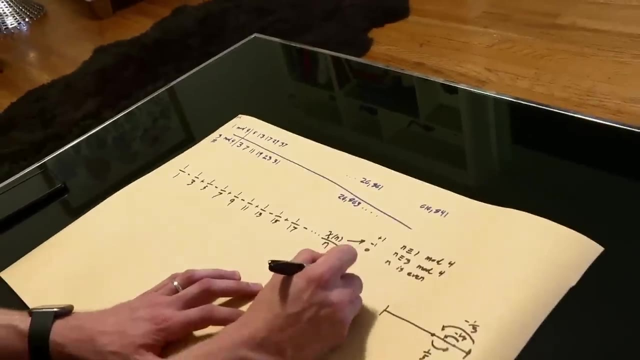 And then if we subtract a seventh, that step was smaller still, And so you're basically bouncing back and forth. You know you're going to converge to something And the value you converge to is pi fourths. That is actually not important for where we're going. 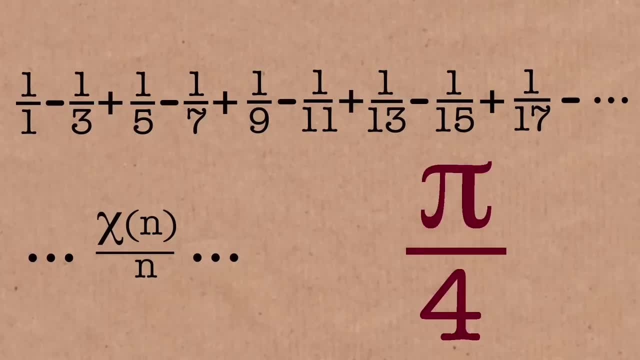 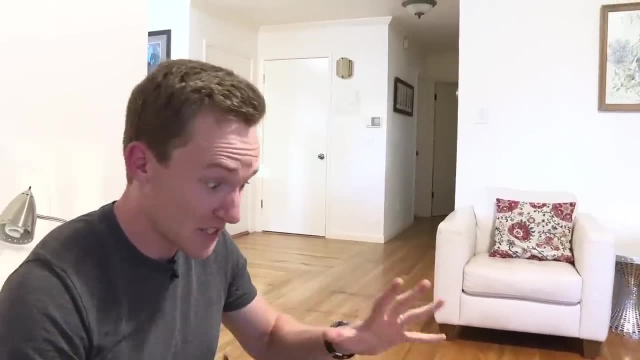 but the fact that it's a number. it's going to be something. Pi. Who doesn't love pi? Pi Great. Right now, pi is almost just like an imposter into our story. It doesn't really have much of importance other than the fact that it's something. 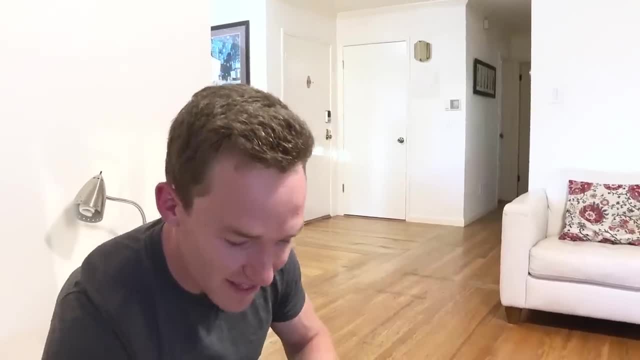 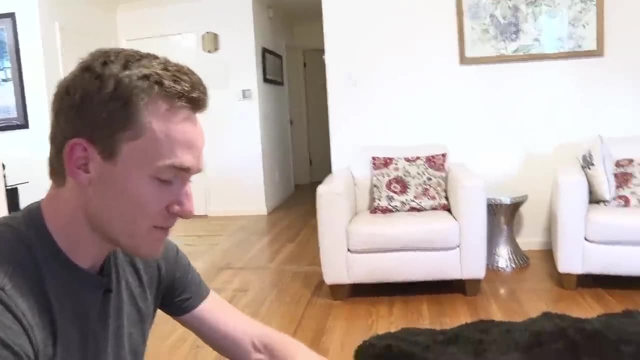 Now the magical fact. the absolute magical fact is the number theorist's favorite way to take a logarithm, And it works like this. We're going to take our series and in order for this trick to work, there's just a couple criteria: the series has to have. 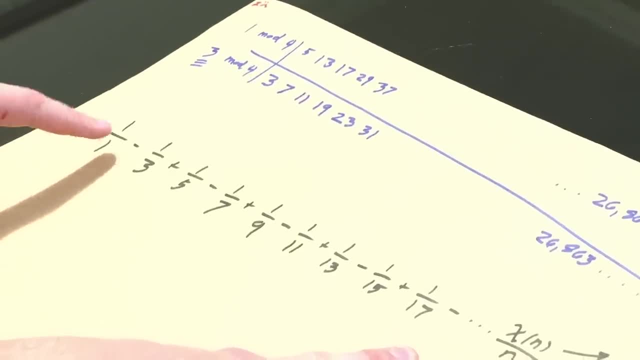 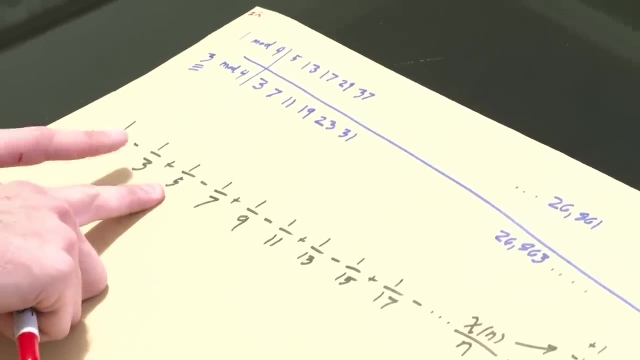 There's got to be a number associated with every natural number, So we might think of zeros for all of the evens here. And then it has to have the property that when I multiply the terms associated with two numbers like three and five, 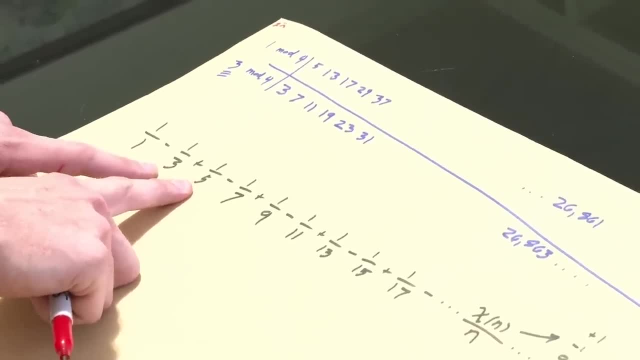 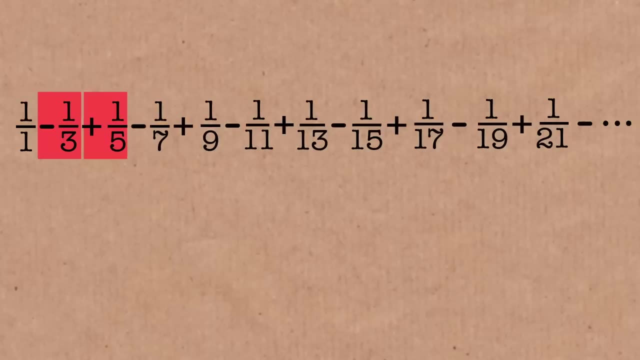 the product of the terms corresponds to the product of those numbers. So in this case, three times five is fifteen and negative one-third times positive. one-fifth is indeed negative one-fifteenth. It's not exactly obvious, but this will hold, no matter which ones you look at. 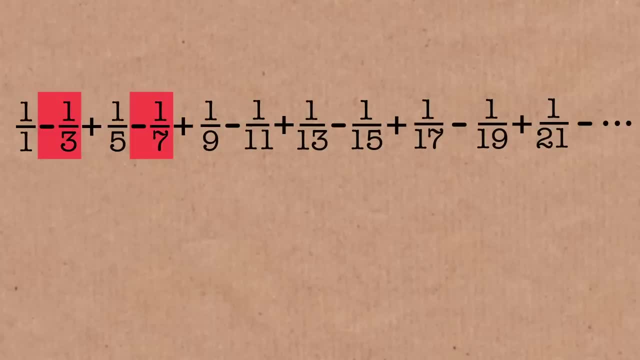 So, for example, if we take one-seventh and one-third negative, one-seventh times negative one-third will be positive one-twenty-first, And if we go up it would be a positive one-twenty-first. So as long as that property holds, you can do this magical thing. to take a logarithm: 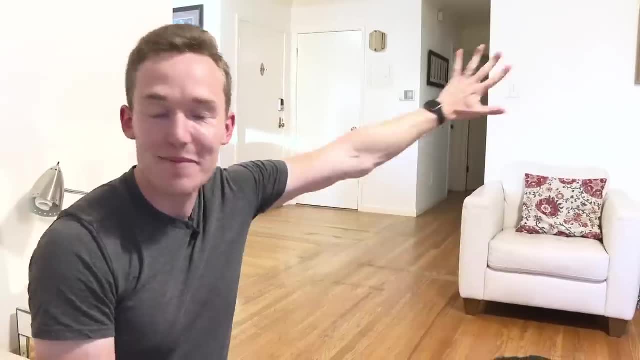 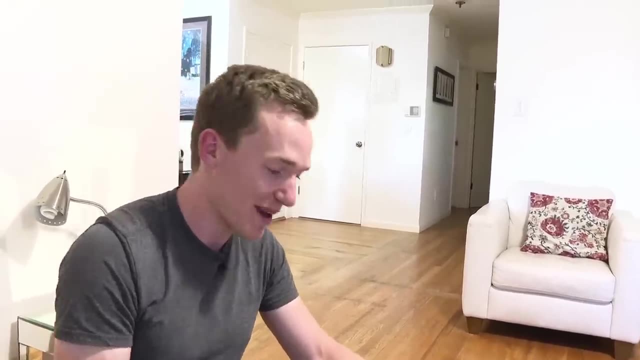 where I'm going to say I don't like composite numbers. I'm going to kick out my composite numbers. If you're not prime, either you're not going to be in the club or you're going to get a strong punishment based on how not prime you are. 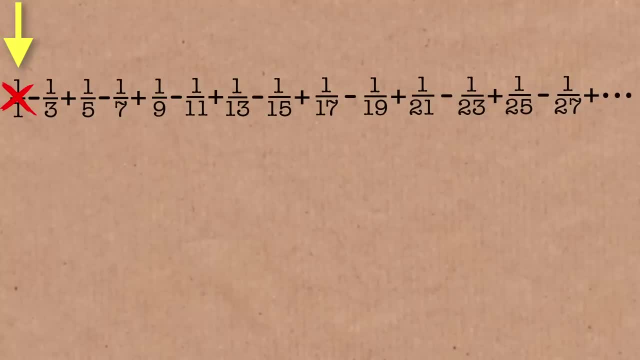 So one: we don't like you. one gets kicked out entirely. One-third, you get to stay, So your term gets to stay. One-fifth, you get to stay. One-seventh, you get to stay One-ninth. we say okay, one-ninth, you're not prime, I don't like you. 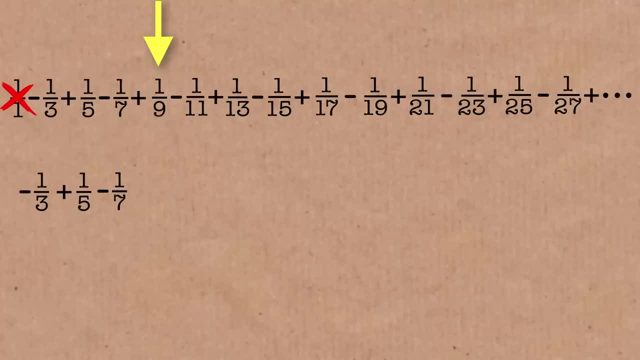 but you're just a prime power. At least you only have one prime factor, So you're not as bad as those dirty composites like six or fifteen. So we'll let you stay. but because you're the square of a prime, we're going to give you a punishment by reducing you by a half. 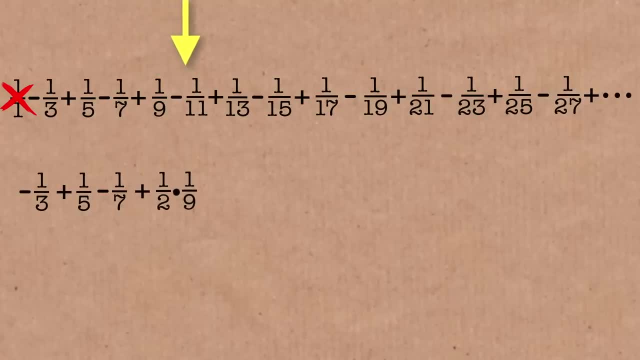 So he gets to stay. but only half is powerful. And then it goes on. One-eleventh, you're prime, you're cool, you get to stay. One-thirteenth, you're prime, you're cool, you get to stay. 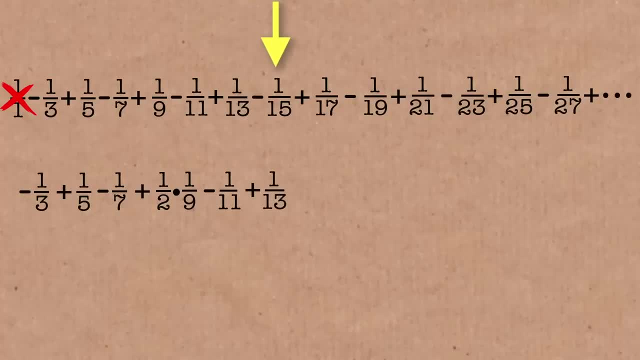 One-fifteenth, not only are you not prime, you have two different prime factors. you're very composite, you're out of the club entirely, And I'll just do a couple more to kind of make it clear. We've got one-seventeenth and notice, I've got two pluses in a row. 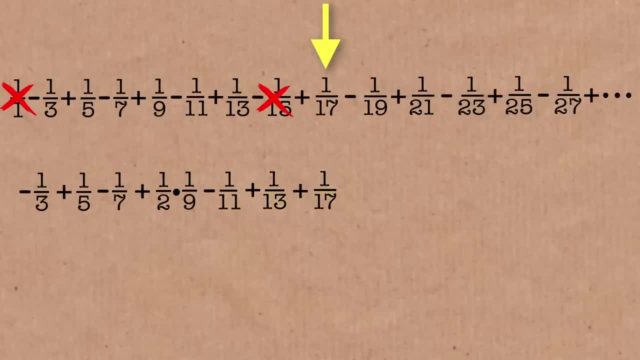 but that's because we kind of kicked out the minus. All we care about is whether this number is one mod four or three mod four. So I'll be subtracting off one-nineteenth. I will also be subtracting off one-twenty-third. 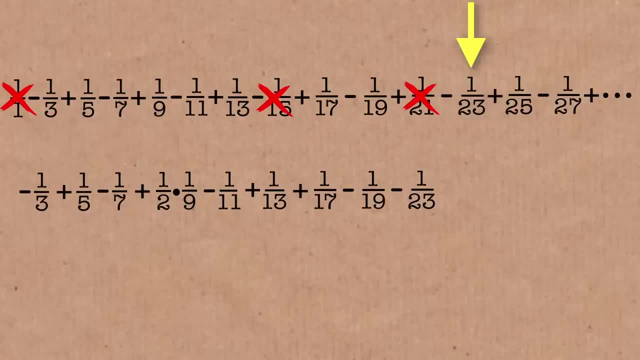 because one-twenty-first got kicked out for having too many factors. One-twenty-fifth, we're going to have to keep him, but divide him by two. Two, a way of saying, okay, you're not prime, but you're just a prime power. 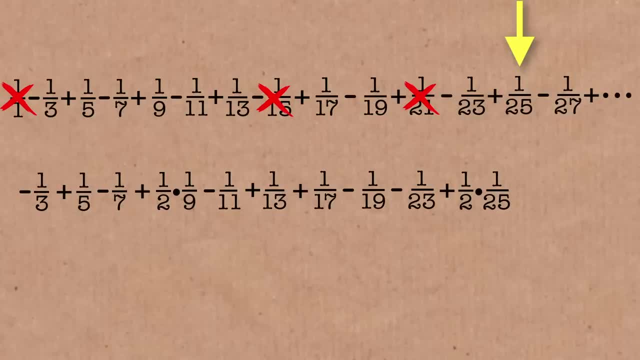 and because you're the square of a prime, you get reduced. And just to make this extra clear, the next one that we see is the cube of a prime: one-twenty-seventh. so I'm going to reduce it by one-third. that gets me one-twenty-seventh. 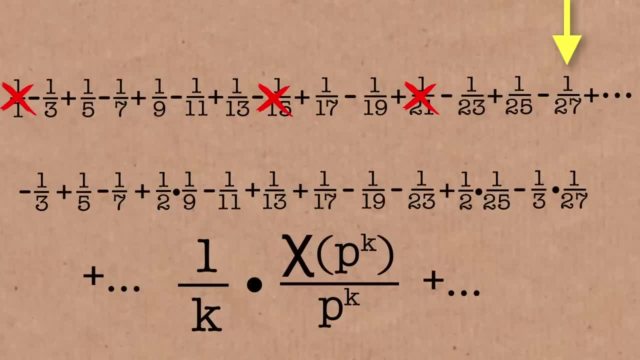 In general, what we're doing here is we're taking one over k times something divided by p to the power of k. where p is a prime number, k could be anything, and we're basically taking this chi function of p to the k, which is just a way of measuring. are you one mod four, or are you three mod four? 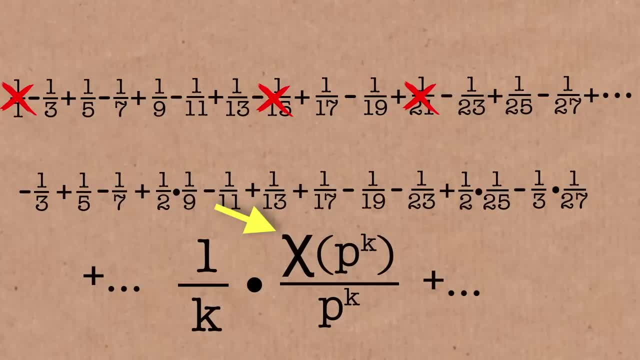 So that might be how you write this in general. So, Grant, if this is some kind of shortcut, it's not feeling like a shortcut, but all right, So it's not a shortcut, it's just the coolest way, because if you 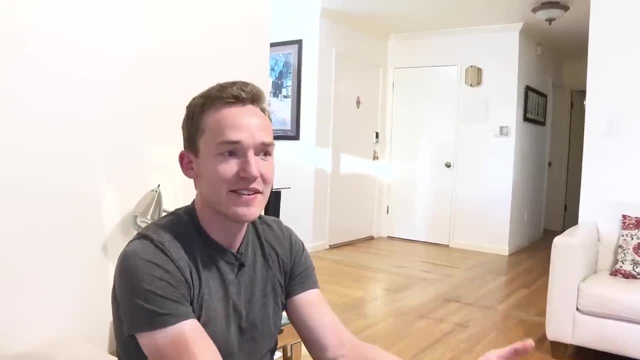 Okay, I do this. I do this completely random procedure to my series and you'd say: what is it going to equal? I don't know? some completely different number that's completely unrelated to the thing that we started with, because you wouldn't. 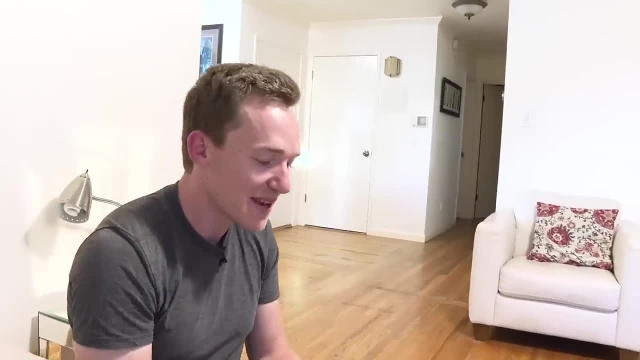 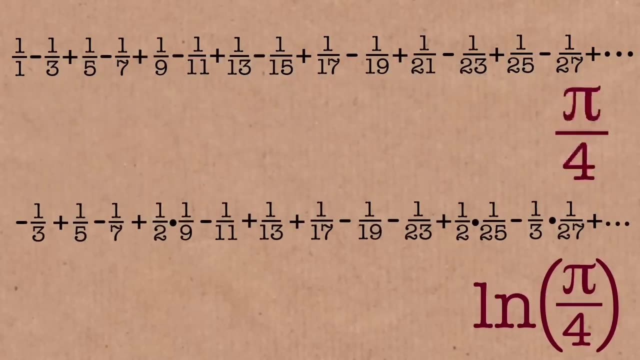 Primes are such a random thing that you're hacking them off at these seemingly random points. you should expect nothing normal to come from this, But the beauty is that what you get is just the natural log of whatever it was before, And we can do this with a lot of different things, actually. 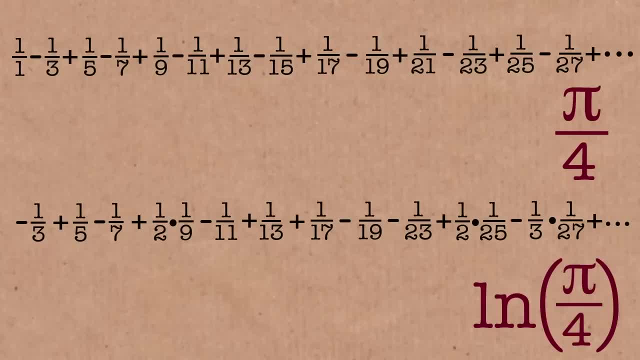 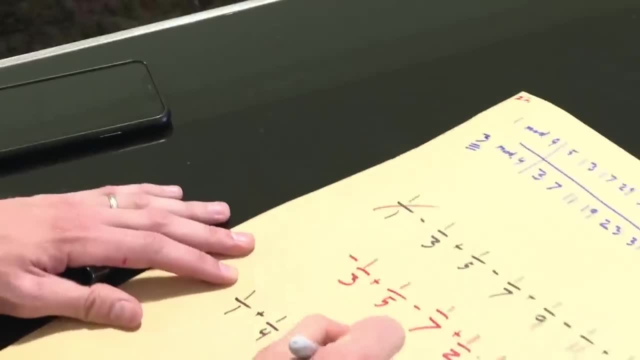 Another famous sequence people might know is if we take one over one plus one over four plus one over nine and we add up the reciprocals of all the square numbers. So we kind of go on and we're always adding up one over n squared. 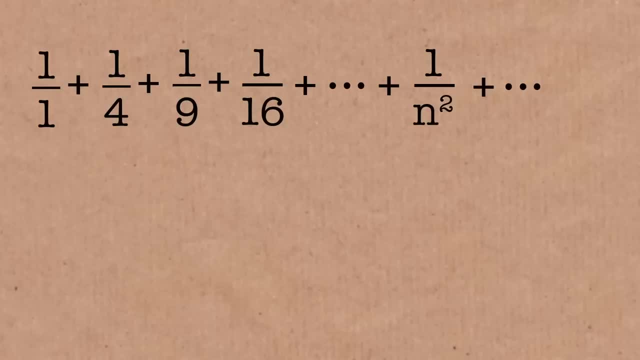 This has the property we care about where. when you multiply corresponding terms, what you get corresponds to their product. If we do the same game, we kick out some prime numbers, we keep the prime powers, but we reduce them a little bit. it'll again be a logarithm. 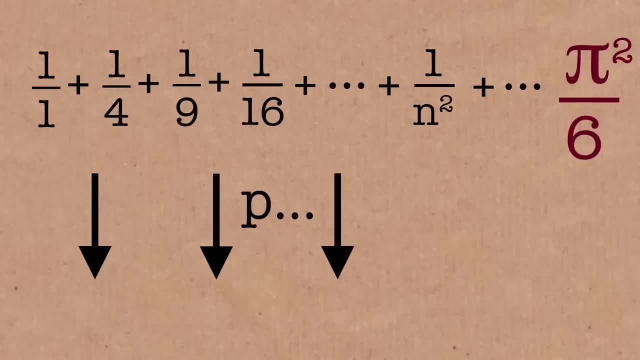 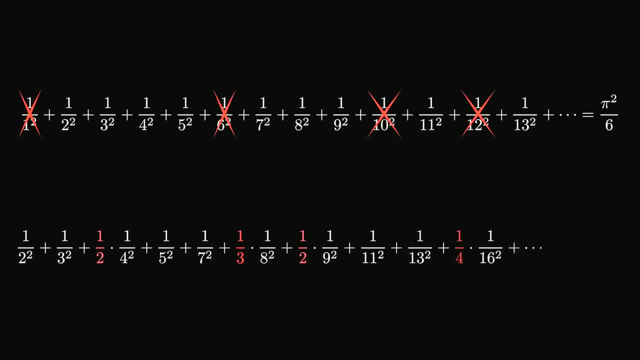 So this sequence happens to be pi squared divided by six, And if we do our whole prime number game, whatever we want to call it, what we'll get will be the natural log of pi squared over six, And so that holds in general, and it's the weirdest possible way to take a logarithm. 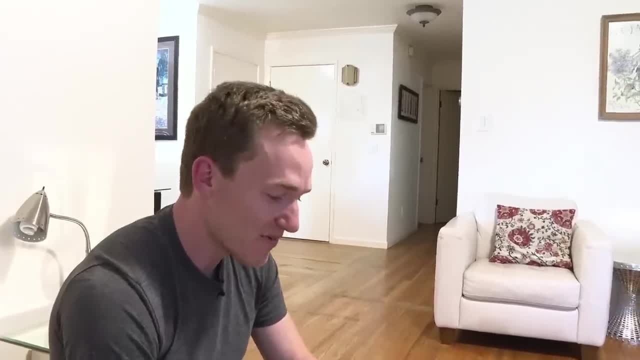 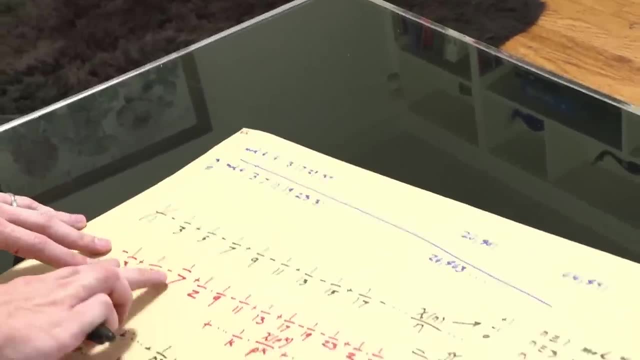 Why am I talking about this? Uh, the reason is that if we look at the sequence that we have here now, we have, uh, mostly primes. We've got some prime powers in there, but it's mostly prime numbers and we're kind of adding or subtracting them. 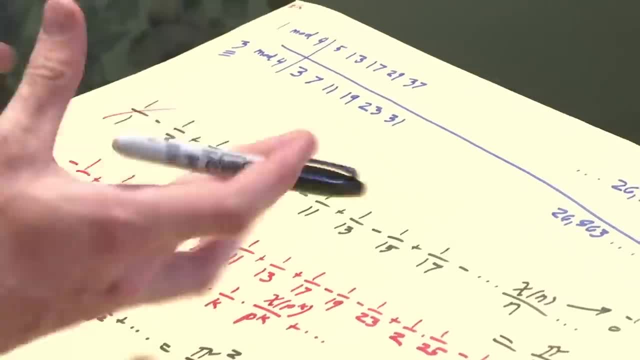 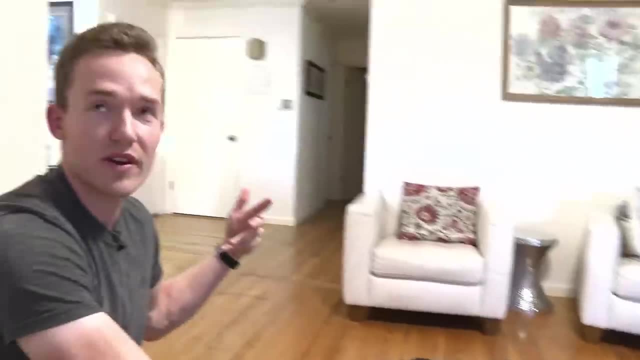 And this might give us a little bit of an indication that if they're to stay roughly, evenly balanced, you know, that would justify the fact that we're equaling some constant Where, if they were systematically way more, that are one above a multiple of four. 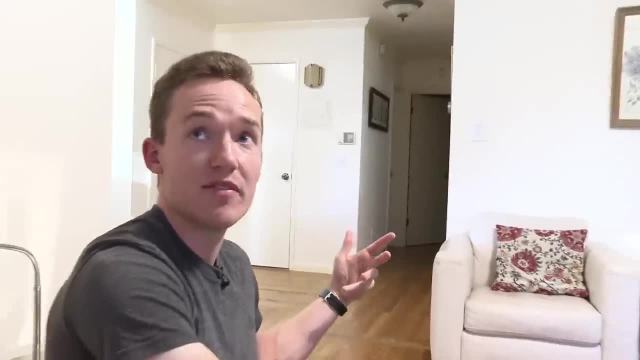 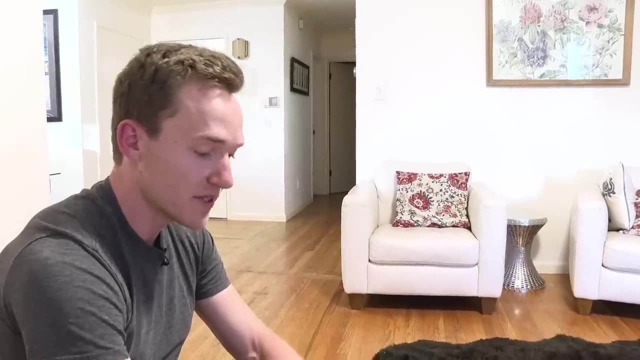 or way more than a three above a multiple of four, the whole series might diverge. Couple other magical facts I'll throw down will be that this series diverges absolutely, which is a way of saying if we changed all of the minuses to be pluses and we just asked. 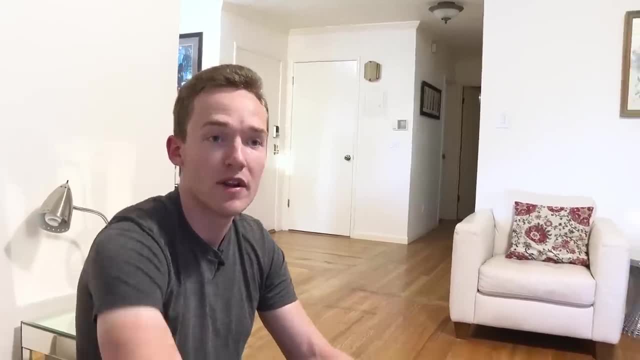 hey, I'm going to add up the sizes of all of these terms. Does that converge to any number? It goes and blows up to infinity, And what that kind of tells us is, if we look at the camp, that are all of the things that are. 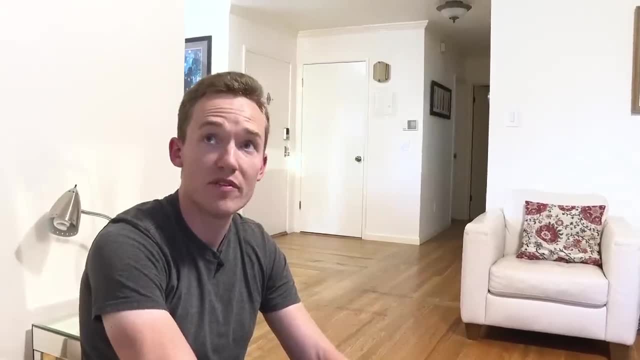 being added and all the camp that are being subtracted. both of those blow up to infinity, And so when we're cutting it off at a finite point, they have to stay roughly balanced with each other. So this tells us two important things. 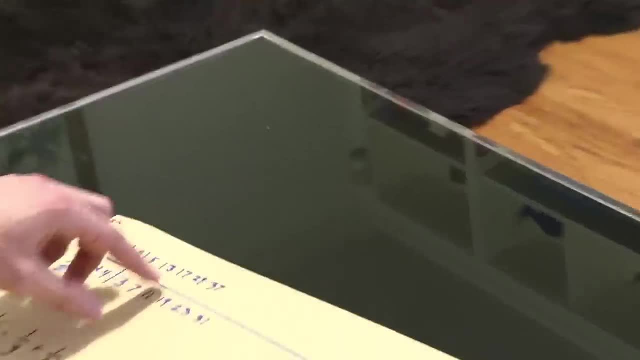 One is why we have a kind of even balance in our race, And it's not that you know, But this was. but you did this with the odd numbers. This is just prime numbers, but it's the same sort of principles. 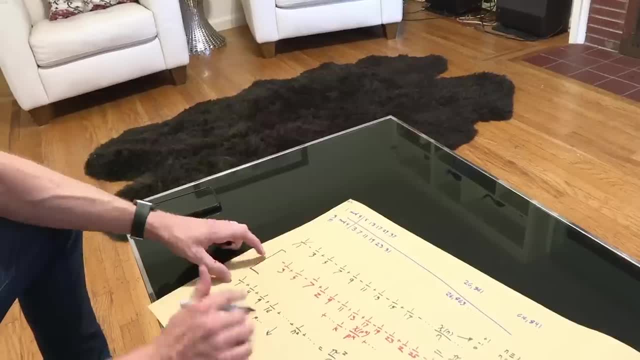 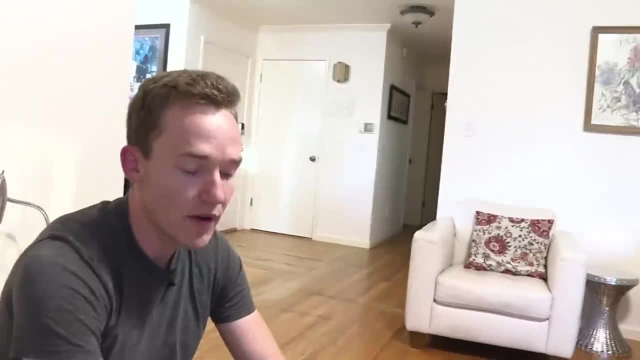 The key equation at this point is to focus on what happens after we do our log trick, where all the stuff that remains in the series is mostly primes. So what I could say is, if we kick out all the prime powers, those, they don't actually amount to that much. 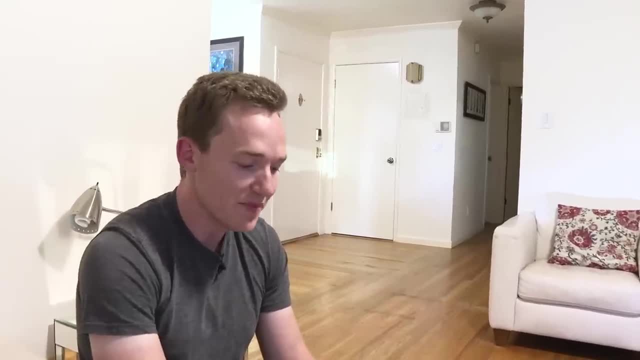 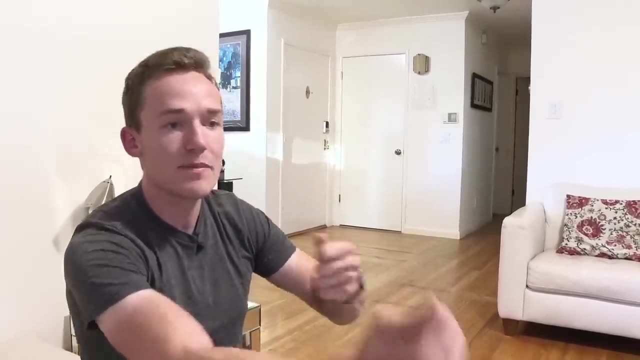 They converge Absolutely. And in fact we could say, if we ignore all the prime powers, we would have this sequence which sometimes you're adding a prime, sometimes you're subtracting it, And because it equals just a constant, just some number, 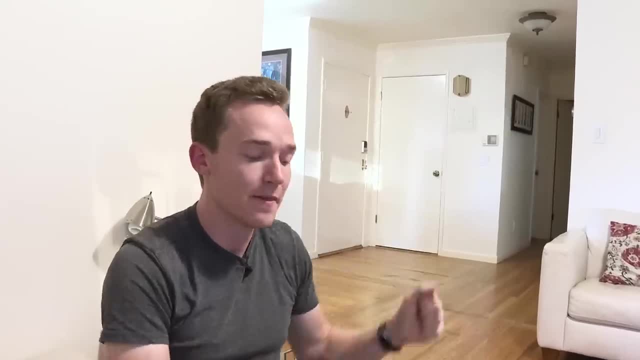 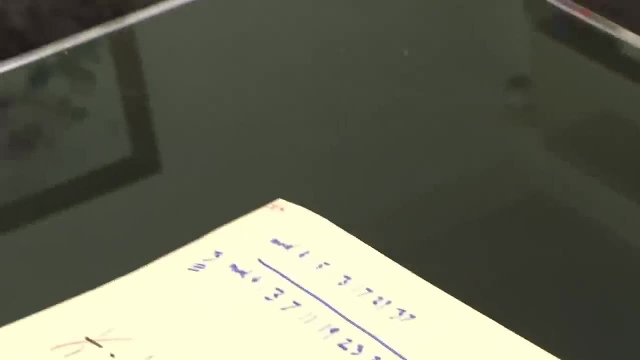 we can know that neither one of those camps blows up much faster than the other. However, all of the nuance for who's winning the race happens when we really think hard about what happens to those prime powers. Here's the like intuition. It is not a proof, but here's the vague intuition for why you might. 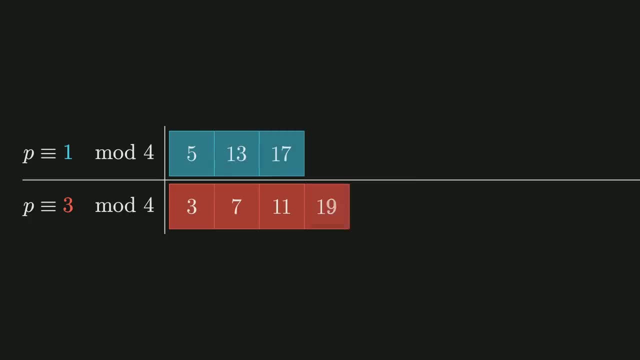 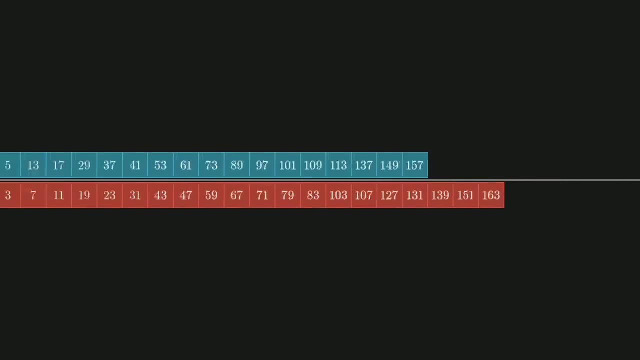 expect three mod four to be winning this race. Even if you didn't start performing the race, if you knew some analytic number theory, you had a strong familiarity with the series. your prediction might be: I'm going to put my money on horse number three. 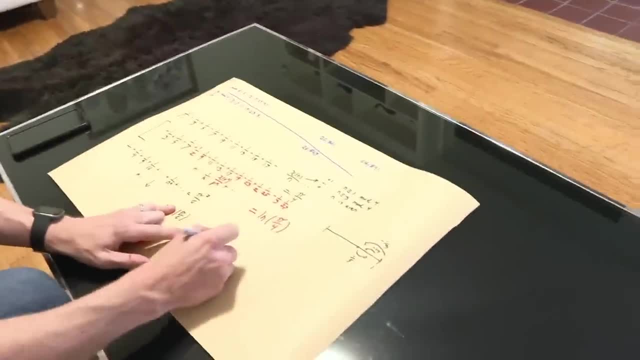 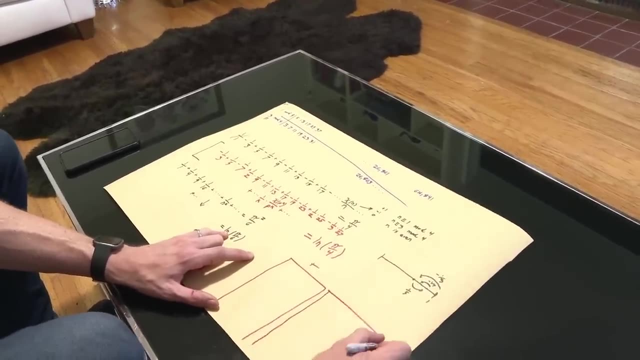 And how do I want to draw this? I'm going to kind of have two buckets here. This is going to be all of the stuff that we're adding in our sum, And then this is going to be all of the stuff that we're subtracting. 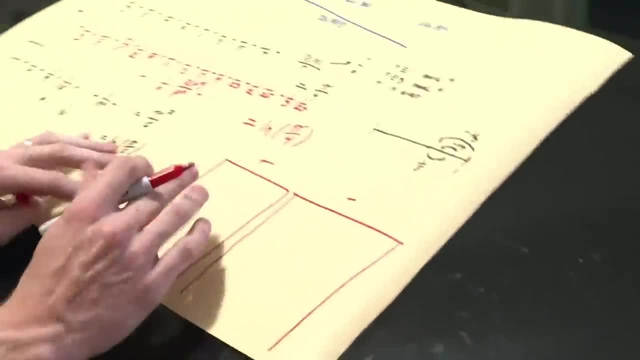 And we're just going to kind of keep. what kind of things are we adding? What kind of things are we subtracting? So the stuff that we're adding, it's all of the primes which are one above a multiple of four. 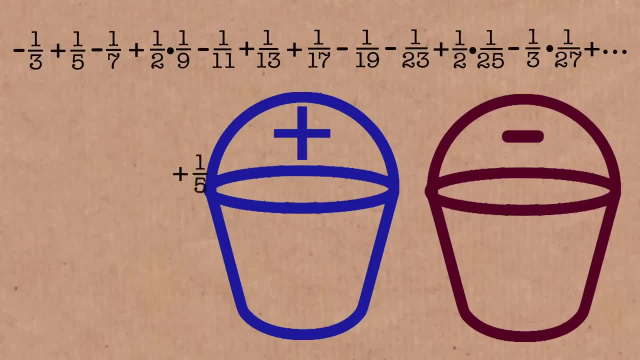 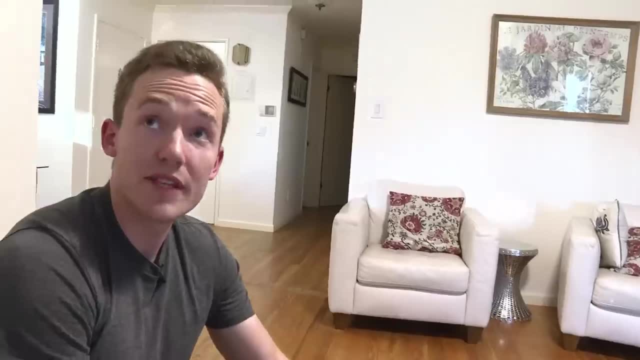 So, or rather the reciprocals of those. So, one fifth, one thirteenth, let's see one seventeenth. These are the kinds of things that we're adding, but there's also some squares of primes that we're adding. 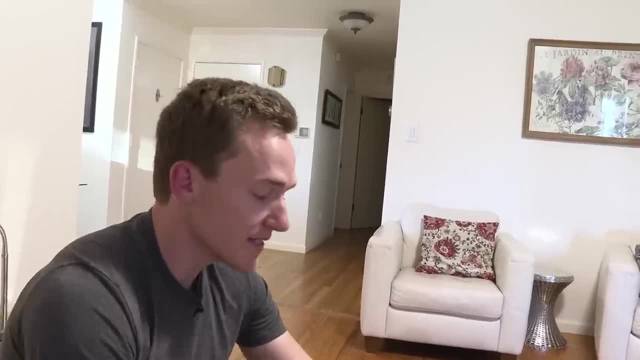 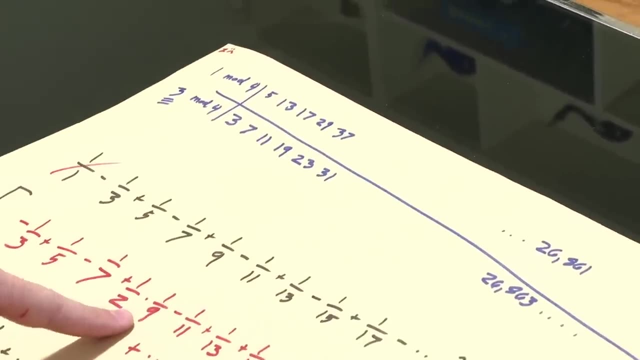 In fact, critically, the square of every prime, because even if you started from someone who is going to be a negative, like negative one third, once we look at the square term corresponding to it, it's something that we're adding. So also. 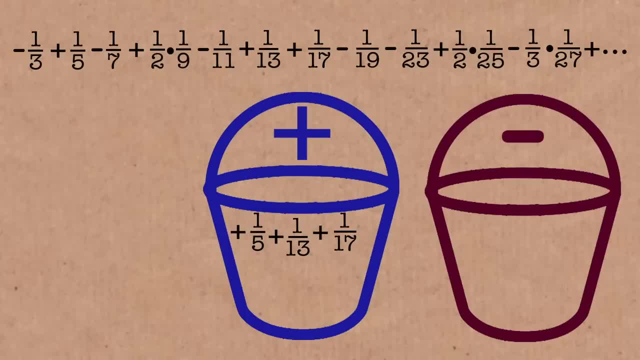 this camp of things that we're adding is you have things like one half of one over nine, or you also have things like one half of one over twenty five, or one half of one over forty nine. So all of the primes are represented here with their squares. 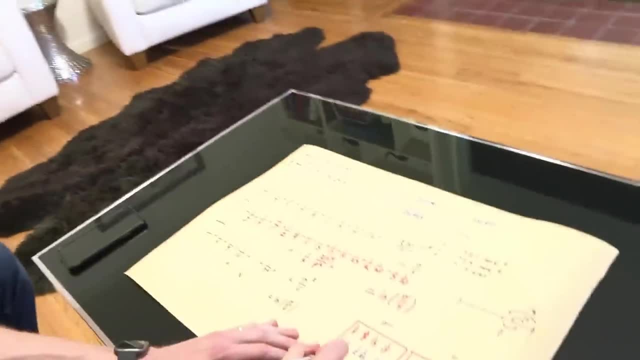 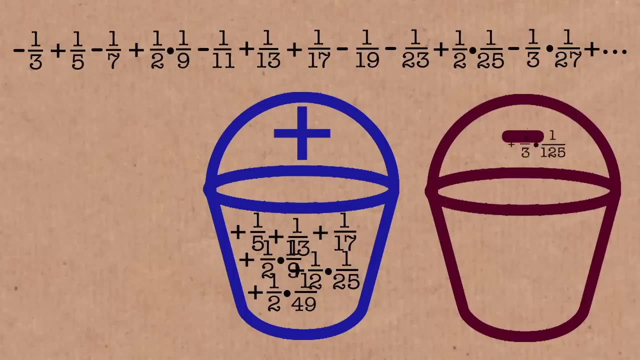 And then in terms of the cubes, those ones are also kind of accounted for, but only the ones which are one above a multiple of five. So, for example, five cubed is going to make it in one over one twenty five, But three cubed is actually something that we subtract. 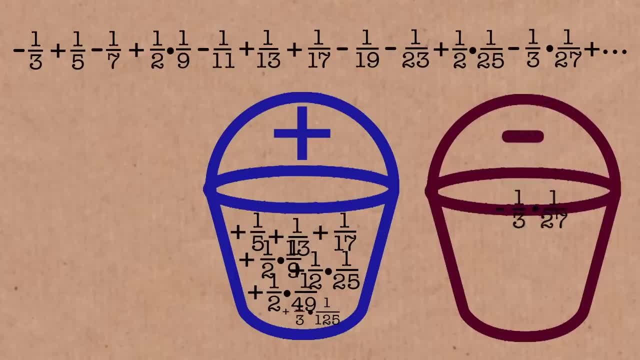 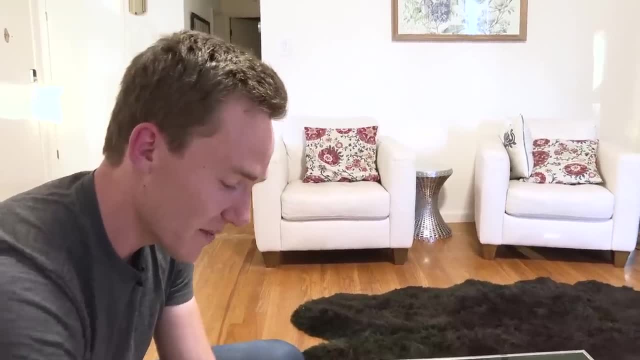 So it's accounted for in the other one, And maybe I'll even write that over here, so that we've got negative one third by one over twenty seven. The point I want to make, I guess, is if we look at this negative bucket, 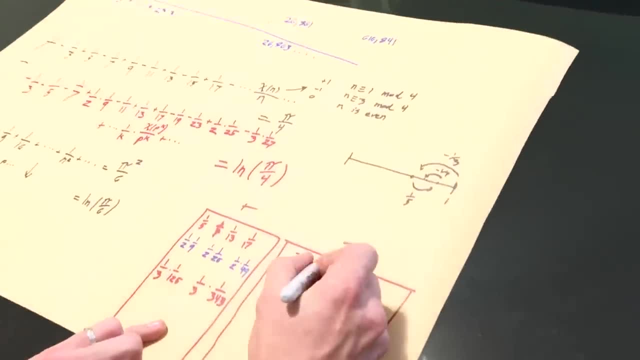 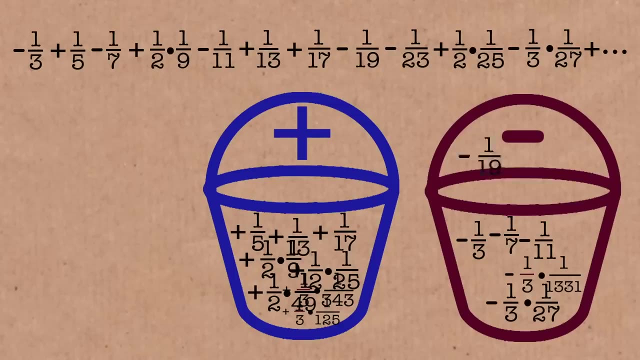 I'll also write up in the top. we're also subtracting all of the primes associated with things that are three above a multiple of four. So we're subtracting a third, subtracting a seventh, subtracting an eleventh. What I want you to notice is how all of the even powers necessarily end up in this positive bucket. 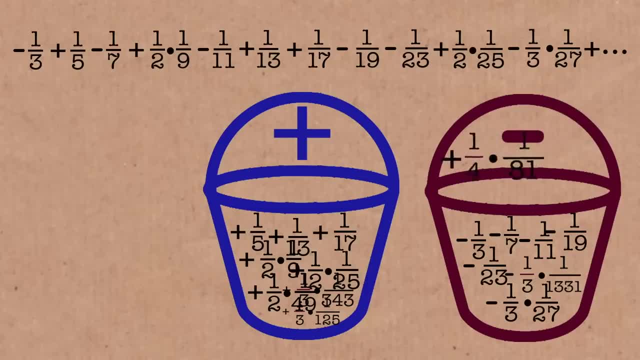 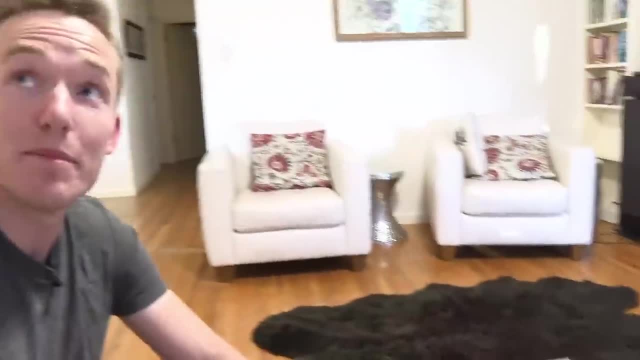 So we also have, you know, one fourth outside of one eighty one. All of the even powers end up here. This gives a bias in some sense in the direction of our adding bucket. So a priori, if we just say, looking at all of these terms, what might we expect? 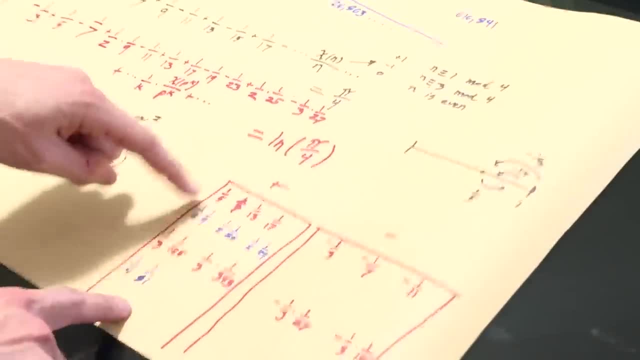 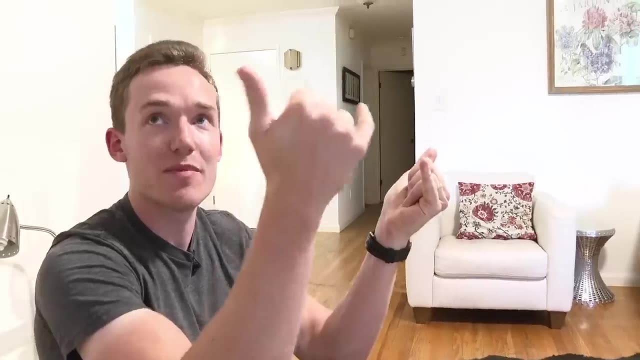 We'd say: well, there's this little bit of a bias for those in the adding bucket to just have more numbers. If there were always the same amount of numbers- one above a multiple of four and three above a multiple of four- because of those powers of the primes that show up here. 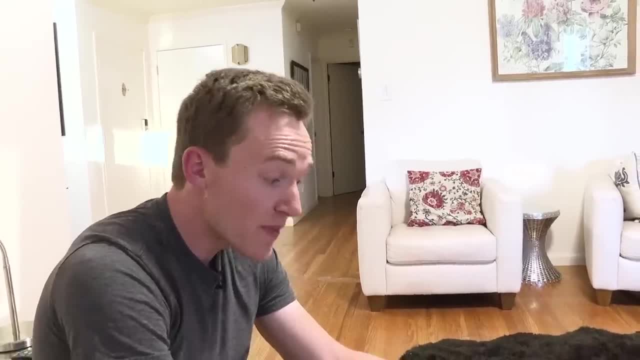 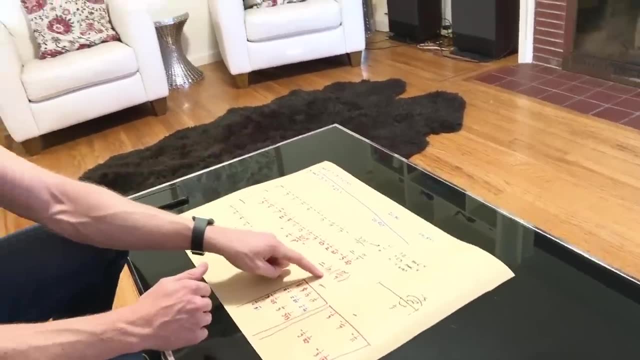 that gives a little bit of added weight to this positive bucket. So if we know that we actually want these terms to be roughly, evenly balanced, in the sense that they're cancelling each other out so much that they get to- I mean, the natural log of pi fourths is a very small number. 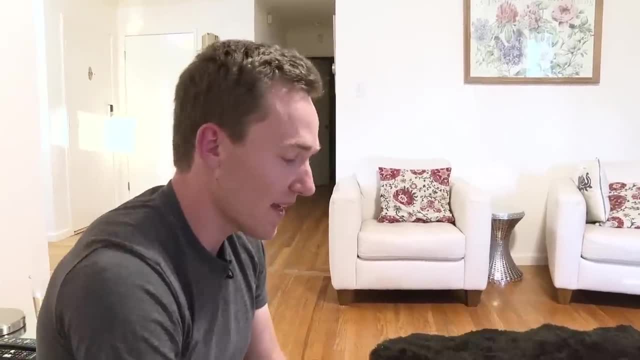 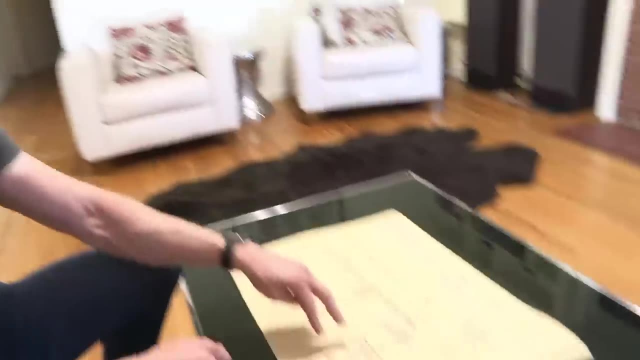 but critically it's a constant. It's not like something that suggests one half of this plus minus bucket is going to tend off to infinity. It means in order to make up for the fault that they get by not getting any of the fourth powers. 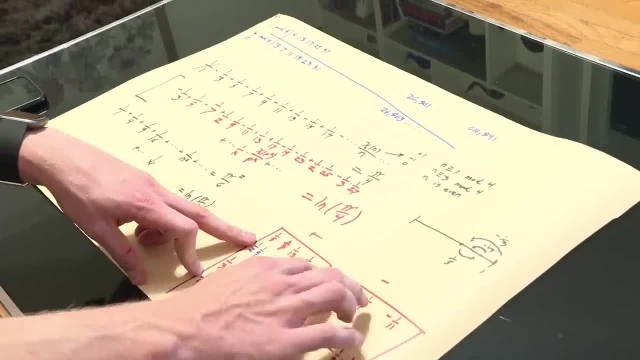 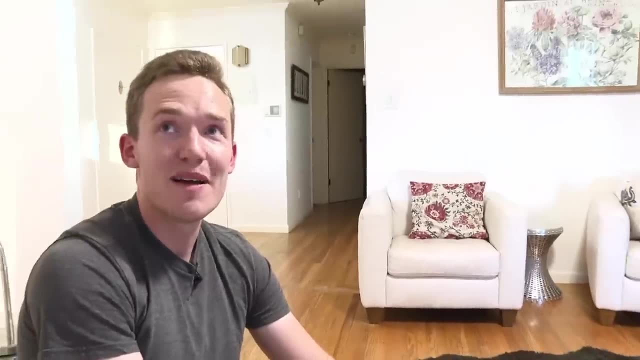 or any of the squares or any of the sixth powers. we need just a little bit more primes to start with, A little bit more that are in this three mod four bucket. Again, it's not a proof, but that's where you might get this little intuition that. 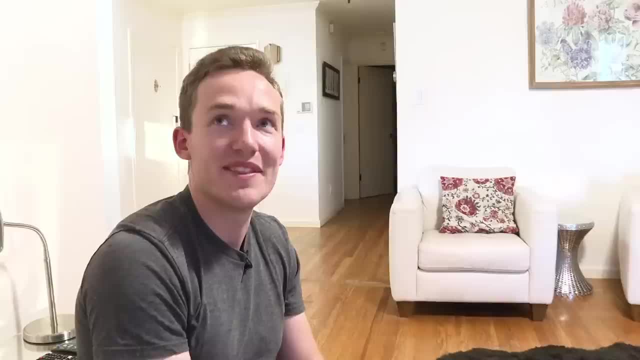 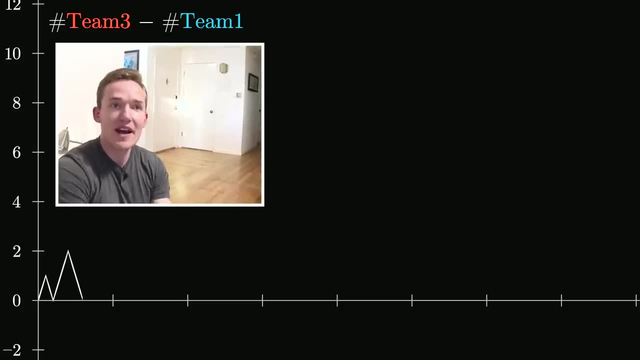 in order for this equation to balance out, you need a little leg up in that second camp. What this would suggest is that there should be a bias for three- team three- to stay in the lead more. There should be a bias for there always to be a few more primes that are mod three. 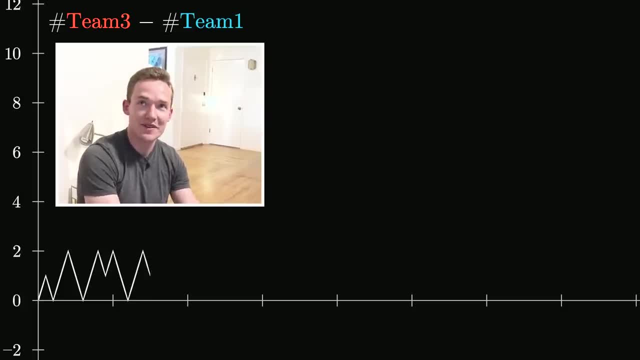 to make up for this imbalance that they get once you introduce the powers. But what you might expect is saying: how often is it the case that they are in the lead If we're watching this horse race, is it the case that after some amount of time, 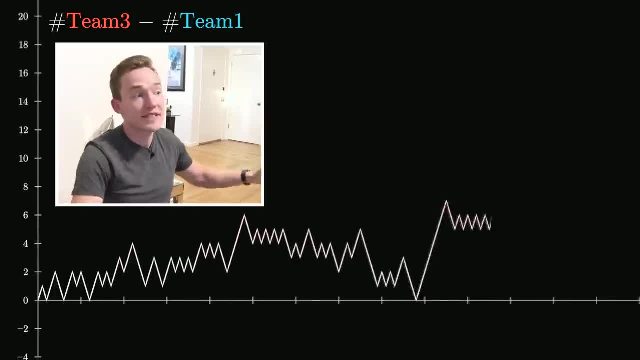 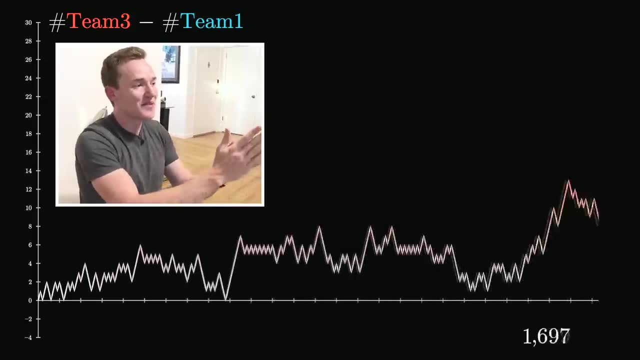 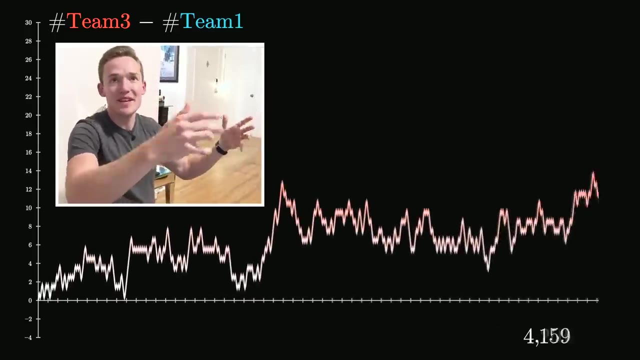 team three always stays in the lead there on thereafter. Okay, that's a little bit strong. The softer consideration, which was the conjecture made, is that the proportion of numbers for which, when you look at everything up to that, the team three is in the lead tends to be closer and closer to 100%. 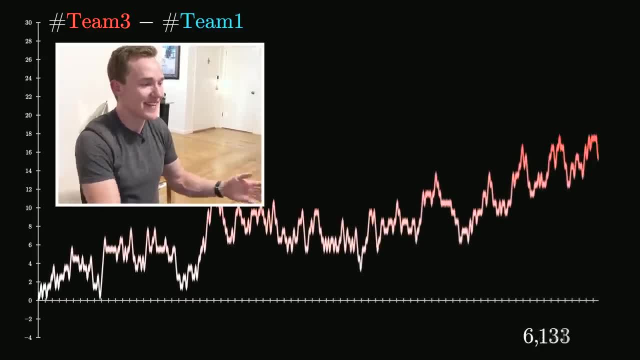 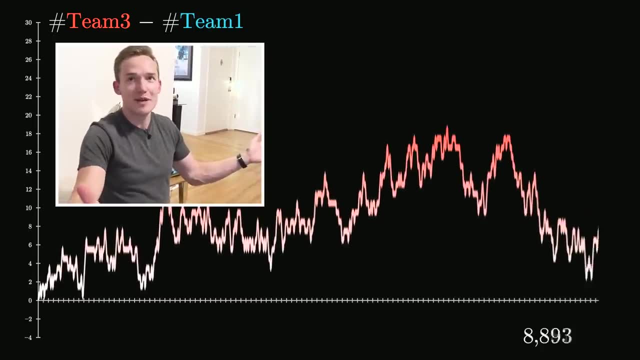 as you look at more and more numbers, As this horse race is proceeding, and you widen and widen your glance, you see various different checkpoints on their track. A vast majority of those checkpoints should be ones where team three is in the lead. Now, interestingly, that's not true. 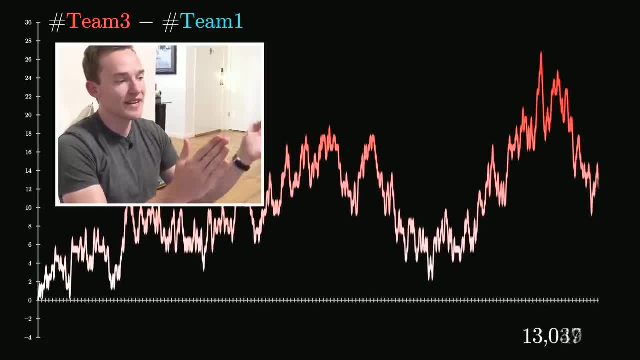 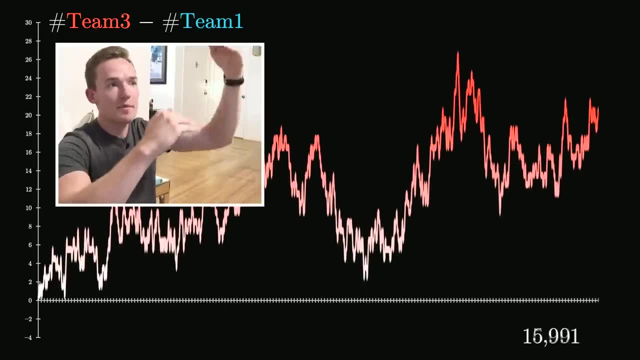 If you look at what's the percentage of numbers where team three was in the lead on your way up, it kind of toggles. It's always very big. It's 99%, 98%, close to 100%, but forever and forever. it just sort of wanders around and it doesn't approach anything. So let's say that if you look at the numbers where team three was in the lead, it toggles. Let's say that if you look at the numbers where team three was in the lead, it toggles. 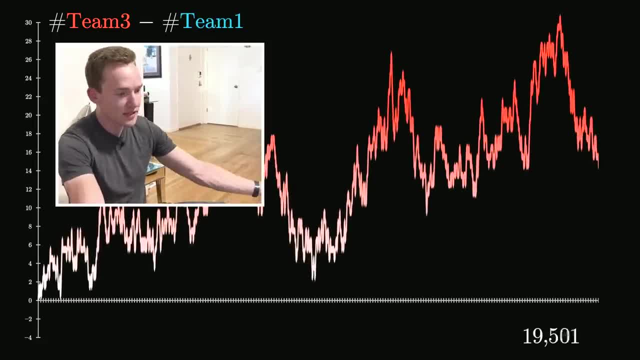 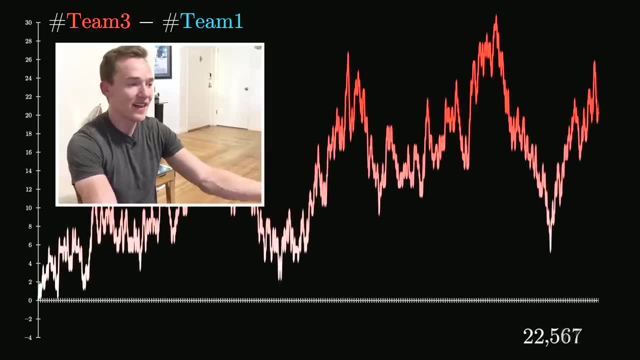 Let's say you look at the first billion numbers, You might notice that as we look at the race up to that billion numbers, 99.5% of the time Team 3 was in the lead, but there were some times that Team 1 was in the lead. 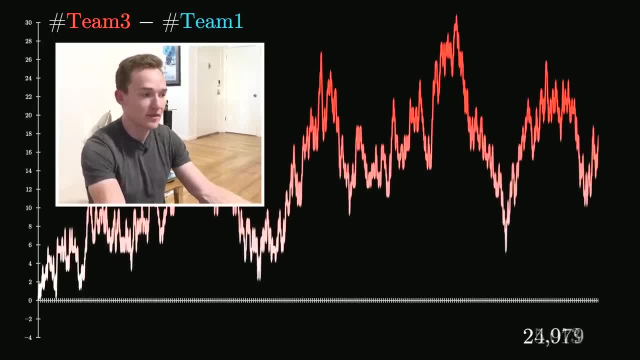 Then you might ask: okay, what if I looked at the first trillion numbers, the first quadrillion numbers You might expect? oh, when I look at the first quadrillion, then it's 99.999% of the time that Team 3 is in the lead. 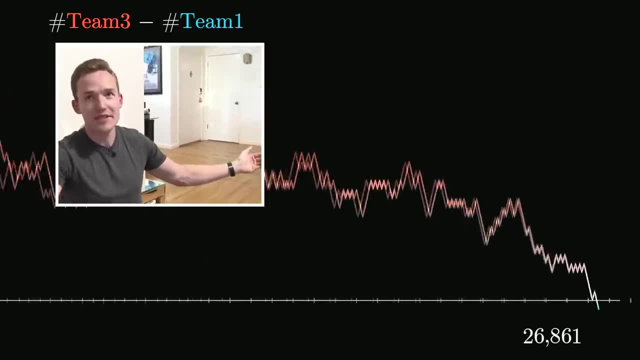 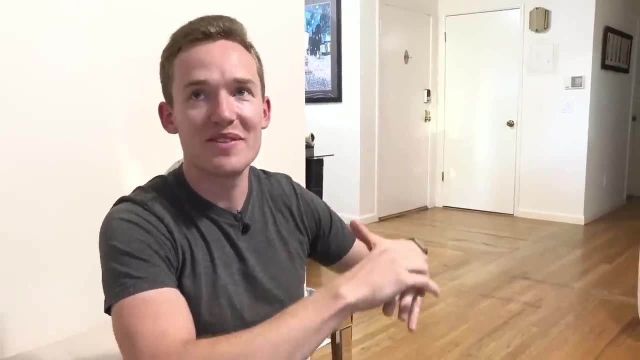 That's not true. As you look at it, then maybe it's like 98% of the time that Team 3 is in the lead, So they do trade off, but there's a clear bias for Team 3, and the question is, how often. 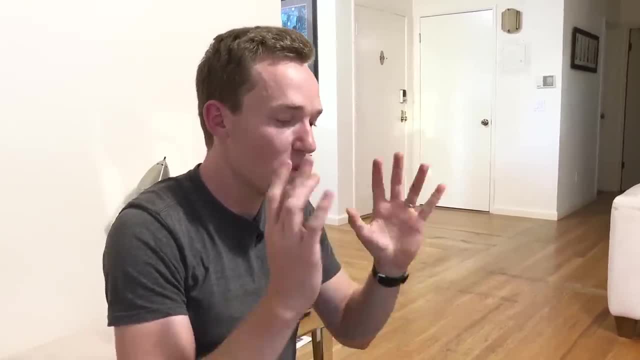 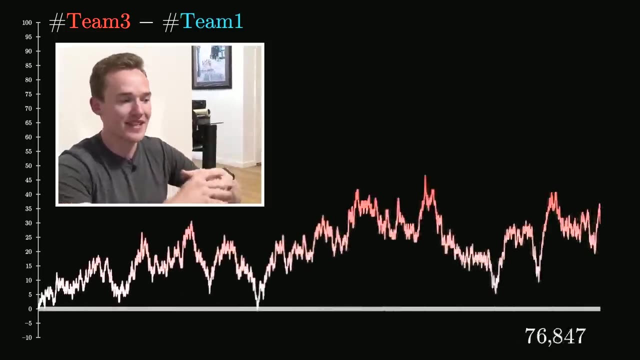 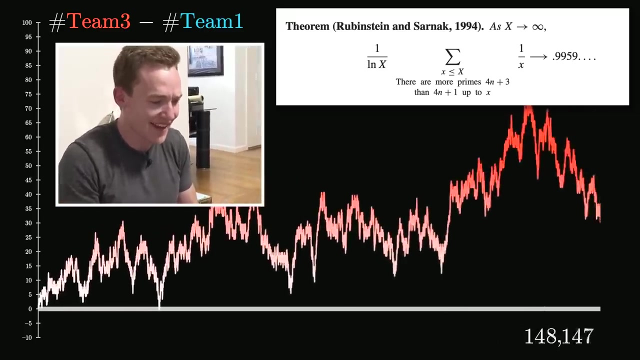 do, they trade off. And it turns out if you measure in a slightly different way. so we're going to change the rules of the race where, rather than counting each prime exactly, you kind of discount them by the reciprocal of that prime For the sake of the proofs. I guess that must have made it easier to prove. 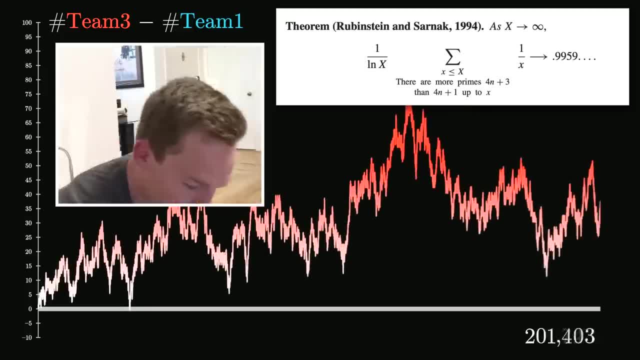 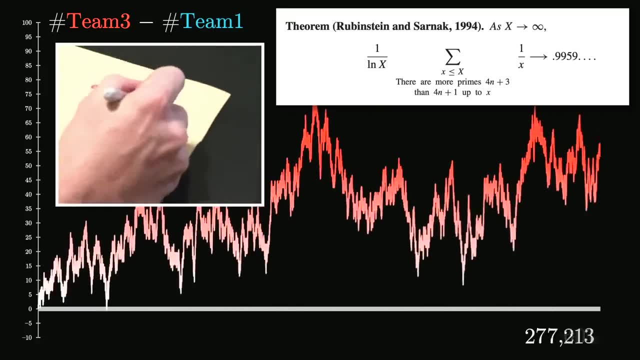 But it turns out that Team 3 will tend to be in the lead. As you look at more and more numbers, it's in the lead 99.59% of the time. So as you look at bigger and bigger numbers, it tends to be the case with the appropriate. 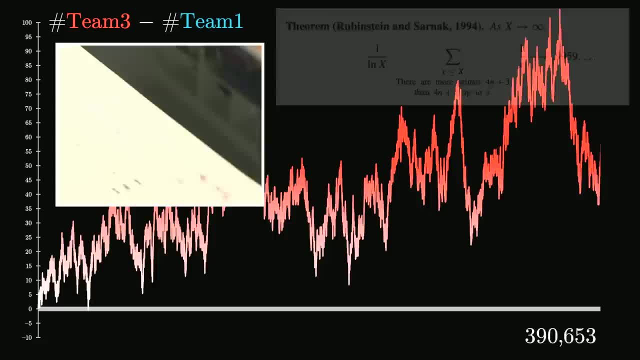 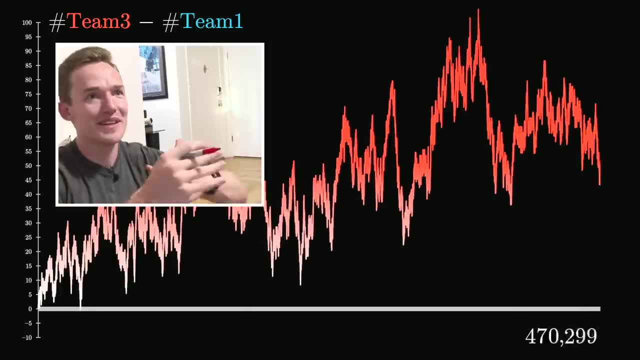 metric that this is the amount of time that Team 3 is in the lead. So it's almost always in the lead, but not almost always in the usual mathematician sense of the phrase, because usually when they say almost always, they mean like 100% or it tends. 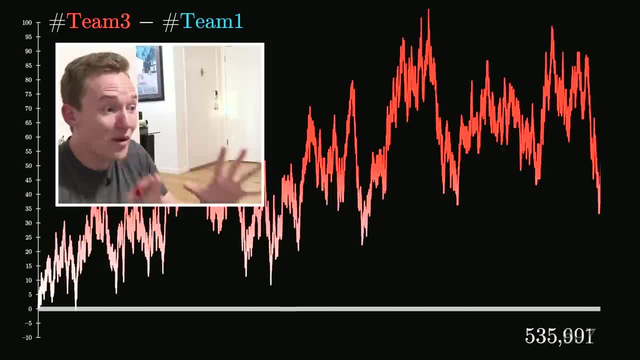 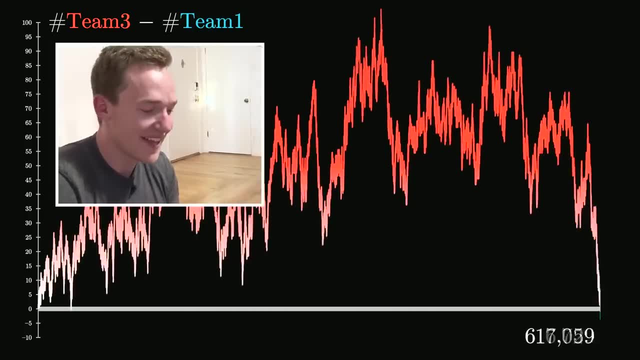 to 100%. So instead it's, in the normal human way of using the word, almost Almost always the case that Team 3 is in the lead, but it is not such a clean fact that it's just 100% or zero. 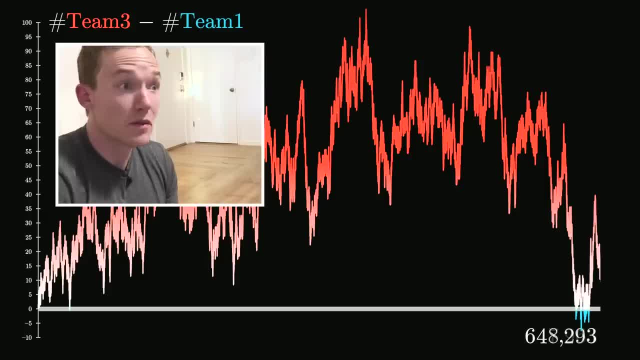 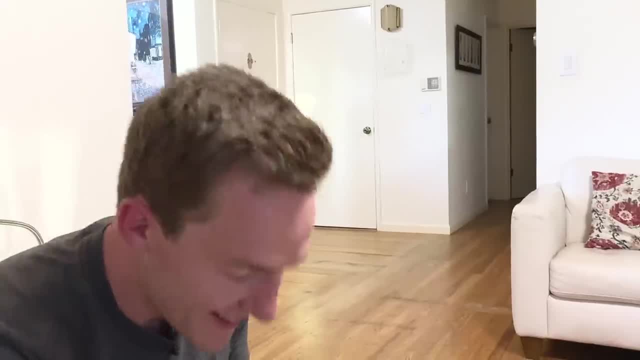 Does it ever get to a point where it will be in the lead forever? No, So no matter where you are in the number line, Team 1 has always got another moment in the front, coming Exactly. Team 1 will always have a chance.